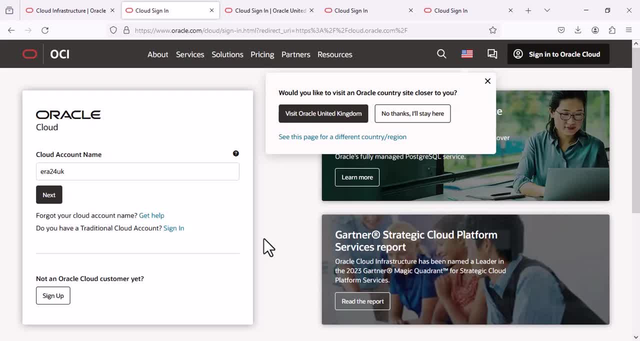 in this video Which will make useful of your free VPS, because I was not aware and I did a couple of mistakes, And so we go to the Oracle one which is United Kingdom Oracle, As right now we are on USA. So once you will click here we will go there. So now we are in oraclecom forward slash UK. 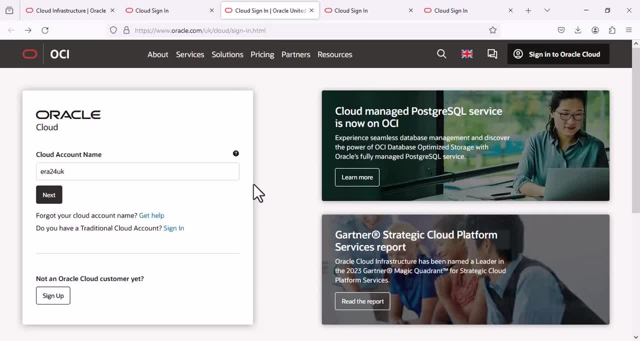 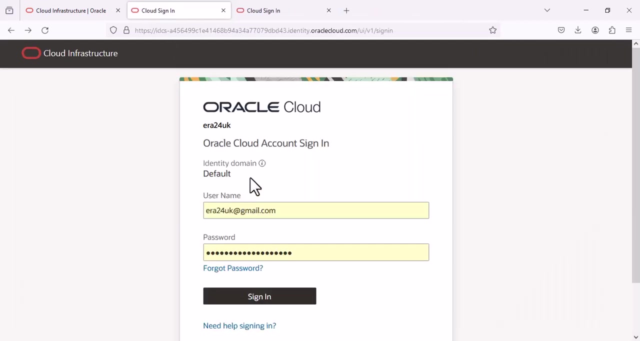 cloud forward slash sign in HTML. once you on, once you are on this page, you can either sign up or just put your username or account name and then click Next. So I'm going to close these all the old one. So we will come on this page once we are going to give our username. then we are on our VPS. 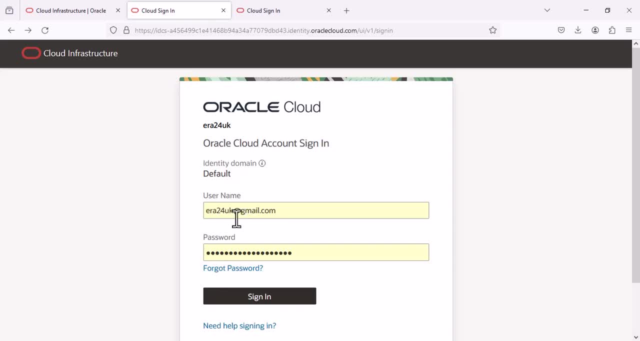 this page now. you give your username or your full email address and your password, then click sign in button. when you click sign in button you will see this kind of page. so now we are going to authorized because when I was setting it up they were asking me to set up the security to do from your own. 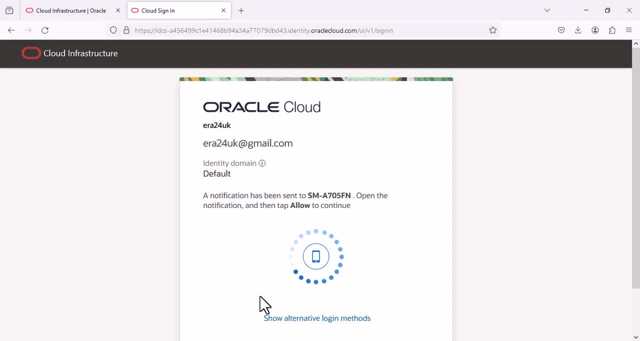 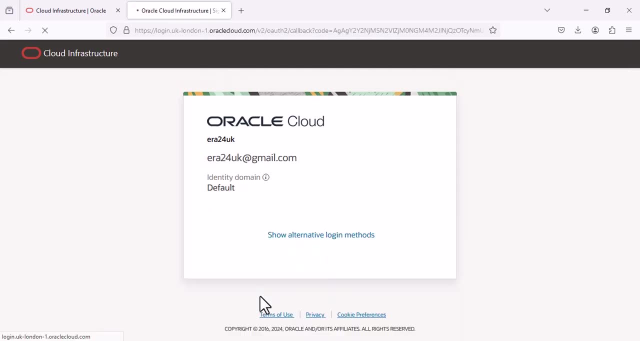 mobile device which I have set it up. now I allow on my mobile phone and it will be working on your screen. great, so I'm going to refresh. okay, I have to sort this out- I don't know what's happening- and continue from there. let's continue once again. you will click on OCI for. 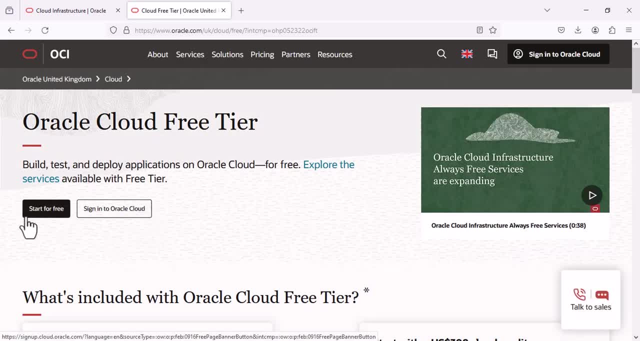 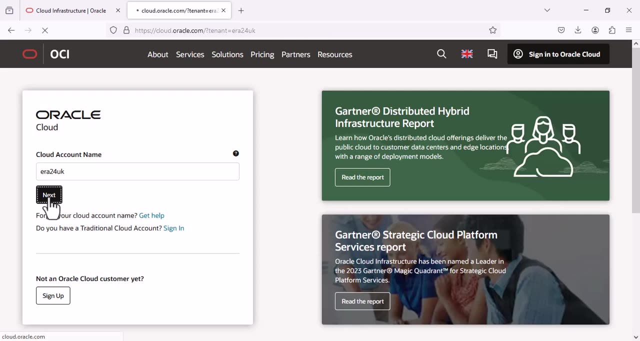 free. and then we are on this page. now we are going to start for free or sign in. so I have already created my account, so I'm going to click on sign in and this is my account name. I click Next and it shows my account number here. 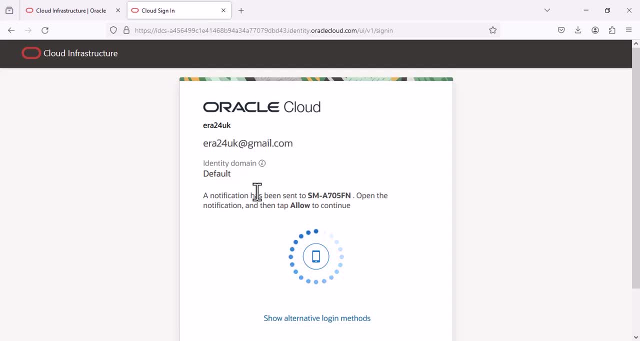 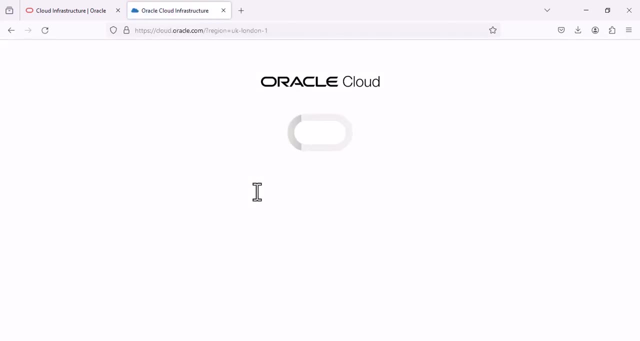 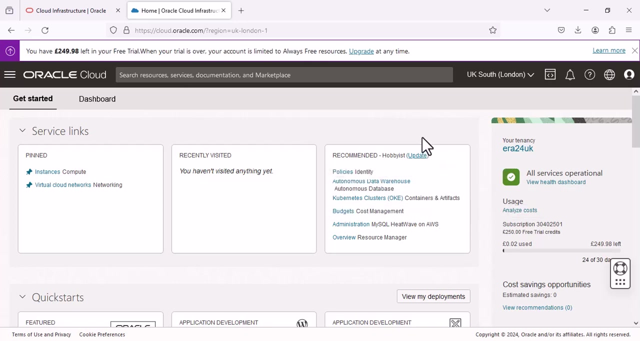 click, enter, enter and it shows that scene. I have already logged it, so I'm going to go through this page now. let's do this: click enter, enter, enter. now again, we are on the authentication. as I told you earlier, I already set it up with my mobile phone. now I'm pressing allow and this should go okay. so I am now in my account afterboat and you will see something like that because you can also check that. you can see that this page is now active so that it will be working on your Bitcoin account. you will see something like that because you can also start your Bitcoin account if you are going to log in here. 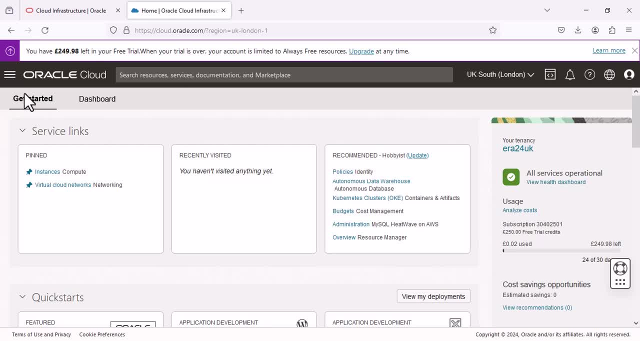 in 2024, the interface. after logging, you will see some something- I mean some- different, because the old version they were showing the dashboard differently. in this one you will see, with some more features and beautiful GUI, as you can see here, get started. they are giving some information which is pinned. 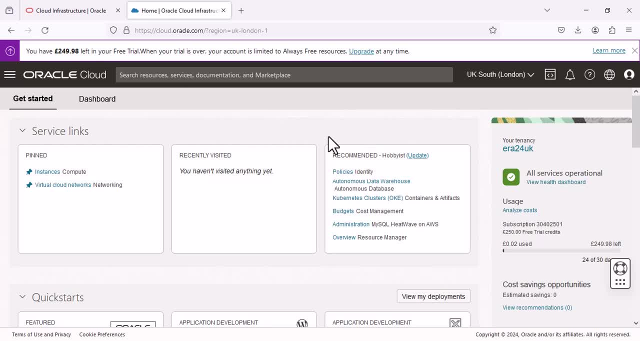 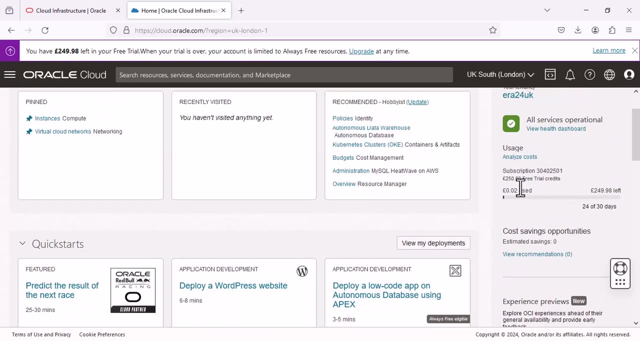 recently visited or recommended. also, you will see ID error 24 tenancy, the all services, operationals, health, which is the health of your dashboard. they are also talking about here the analyze cost subscription and this free trial credits. this and I have used two pens. I don't know how, when. 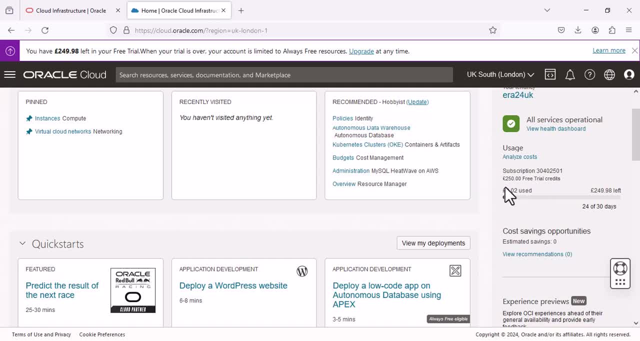 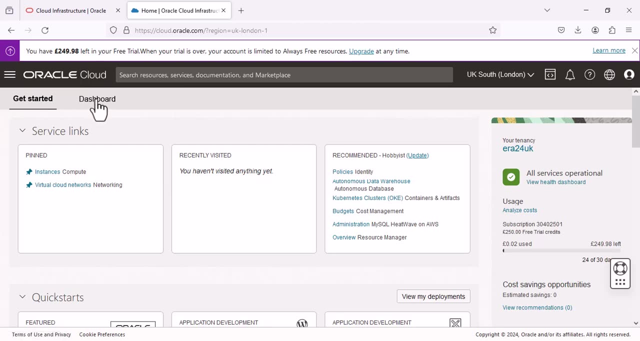 they are giving me free servers, but somehow they have showed me here that you have chopped. I mean, I have used something and I have to pay two pens, and so I'm going to show you what we are going to do. I'm just going to click on. 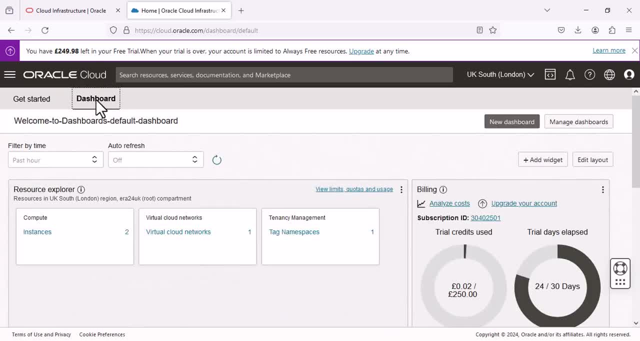 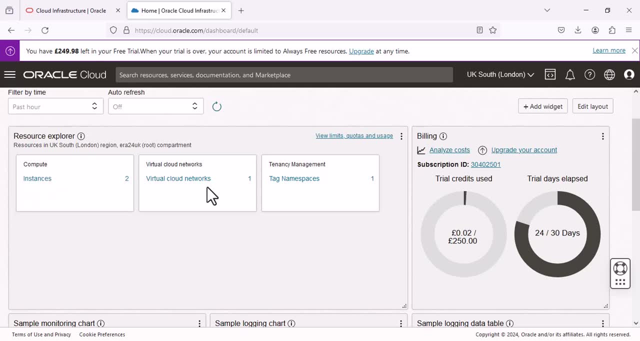 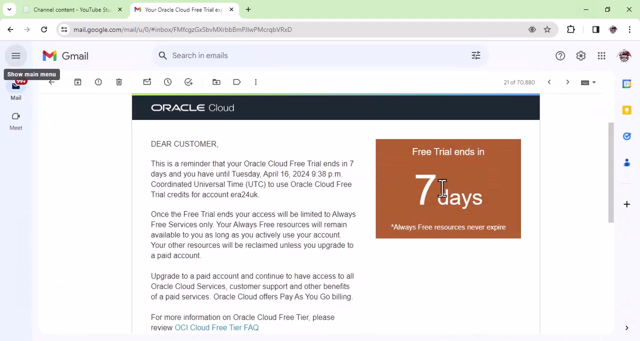 dashboard on dashboard, you can see in instances, virtual cloud networks tagged namespaces and your use credit and trial period. yes, actually I have received this email that I have got only seven days left and I never used their servers because I just tried to create the instances. but the thing is, as I saw in other videos, that they are offering 16gb and 4gb RAM. 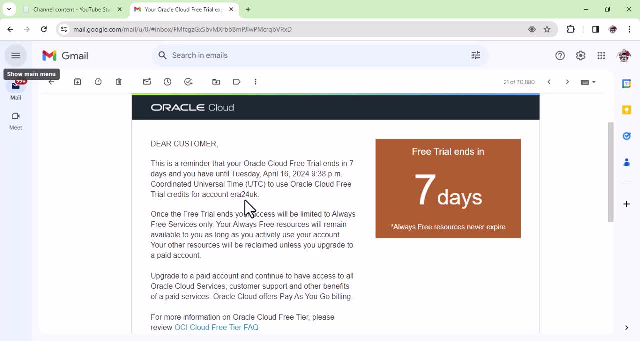 this is all false because once you are in your region- as I am region United Kingdom- I didn't feel good because this is, I feel, third class. they are giving very minimal resources which you will not be able to use. I think. just good for practice, one, yeah, you can say, but you cannot use for your websites or for your 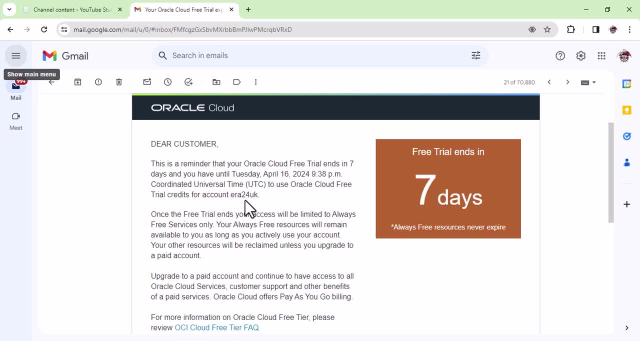 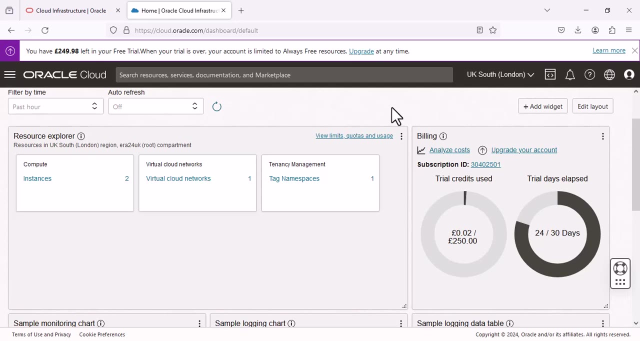 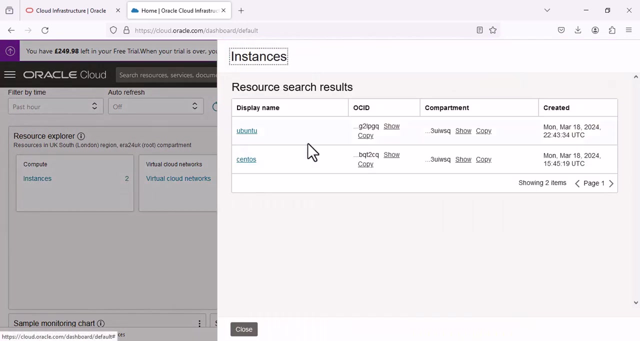 whatever you need to do with your servers. just for practice, yes, but you cannot install whatever you want. so let's continue with my server, which I'm going to close today, unfortunately, because useless for me. I I created two instances. I show you here we are, and that's. one was Ubuntu, another one was 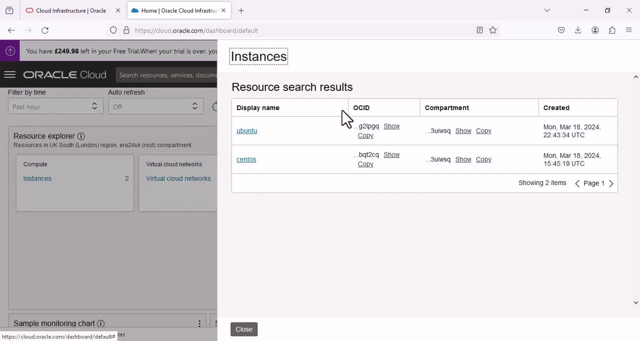 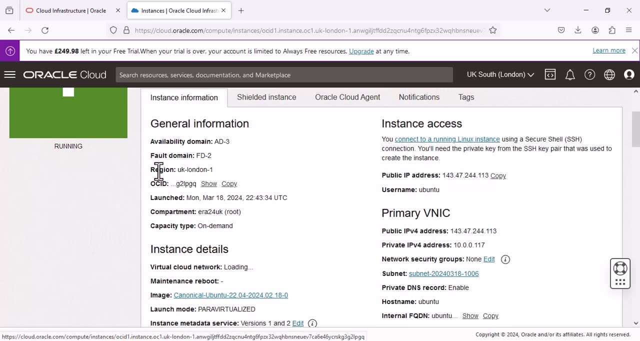 CentOS and I will show you the specifications. let's see so here you can see the region is UK one. okay, this is the domain. they have given me a d1, 82, 83, which is I. I haven't got any other choice to take a d3, because if I take a, 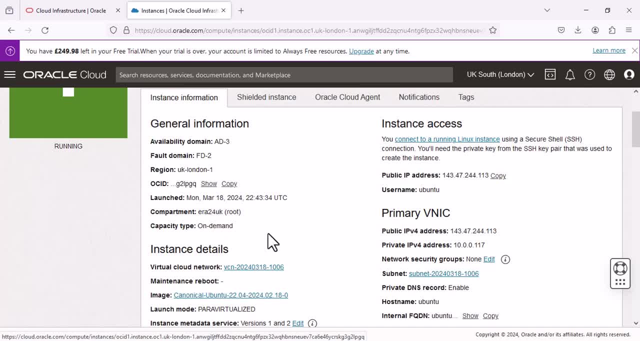 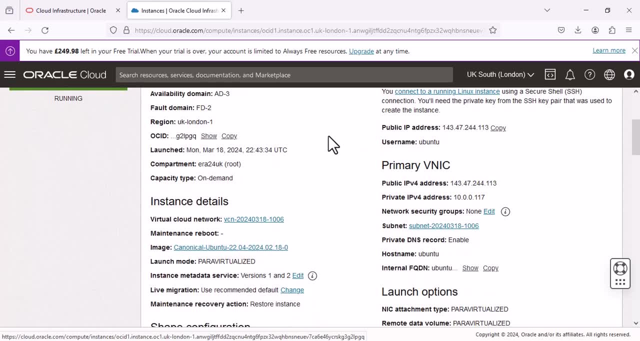 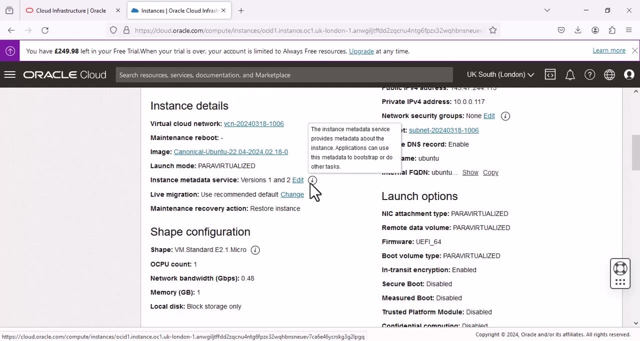 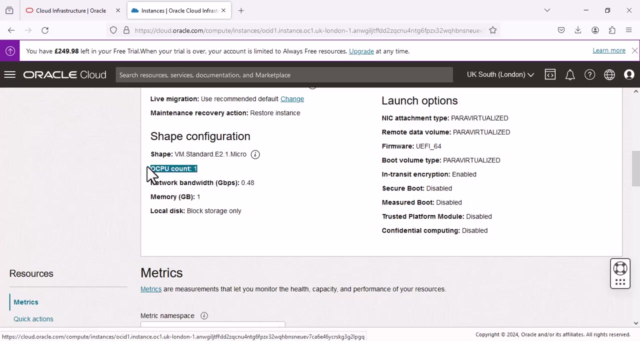 d1, the, the Ubuntu is not allowed. on that one I've got very good kind of headache, you can say, because I'm just trying to install Ubuntu and they don't allow the same thing. they have given me only one, one or CPU, which is one CPU, and 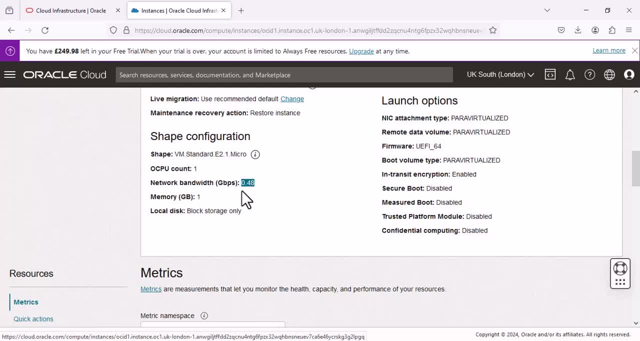 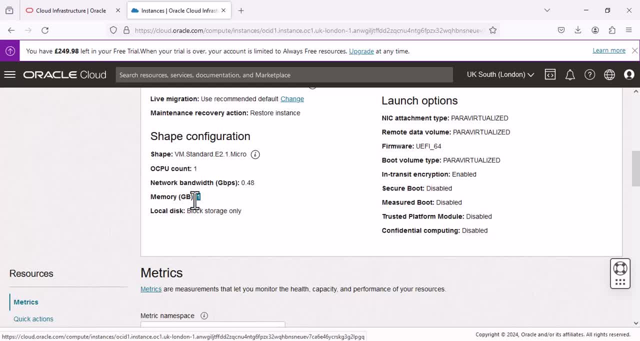 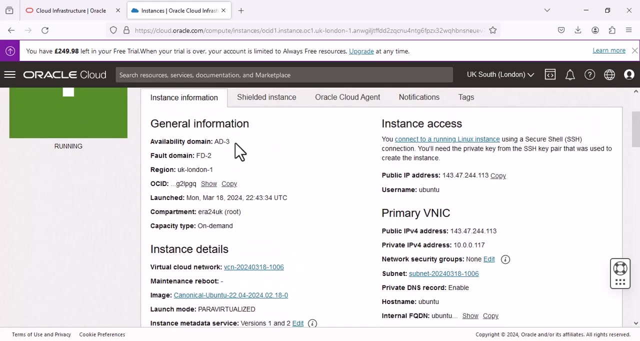 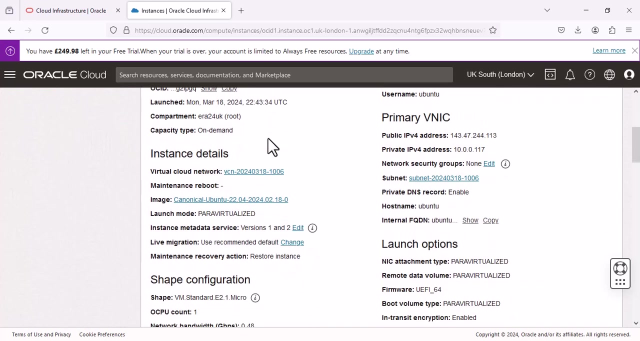 least people are creating in their own videos. they are showing: yeah, you can create, create, create this kind of server, this that kind of server. but that's not true, because they are giving you whatever they want to give you. and same thing, you can install the operating system not on every available domain or the server center. so this was the first server and you can see the. 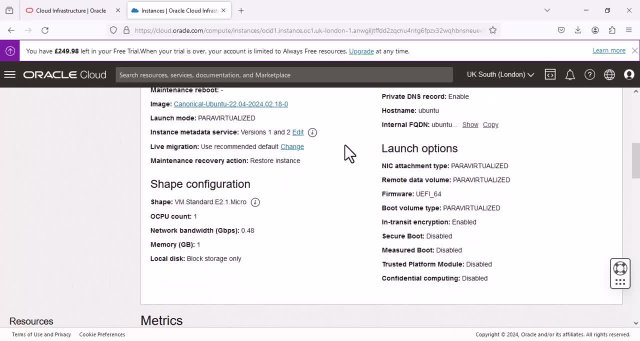 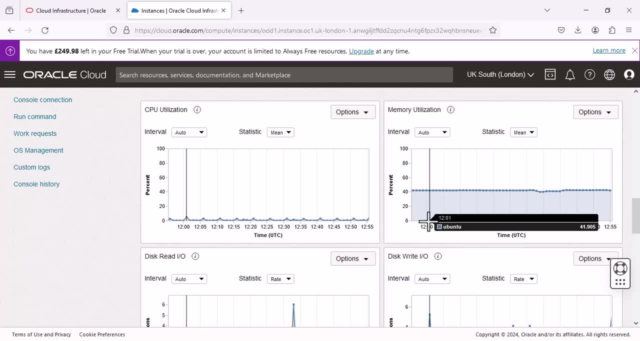 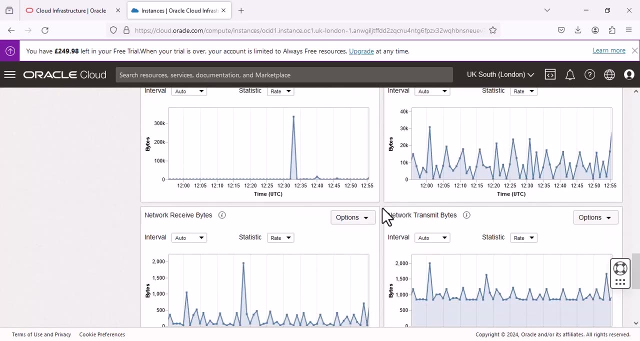 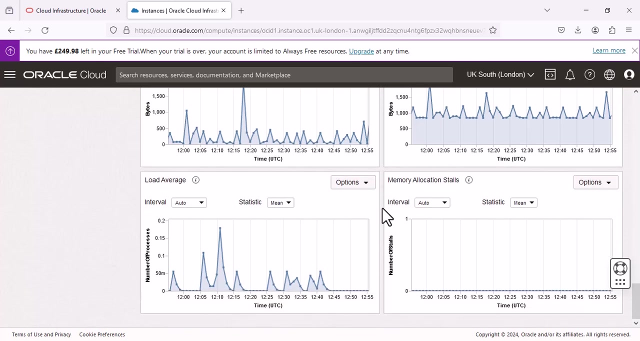 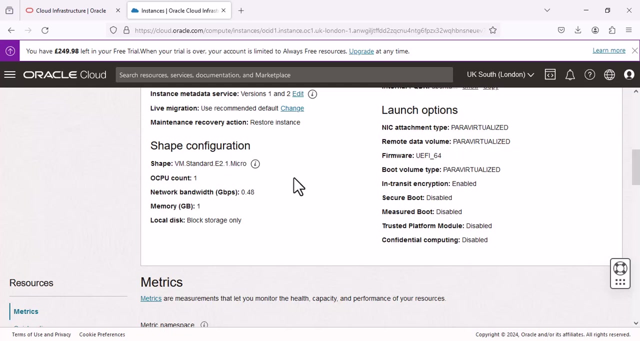 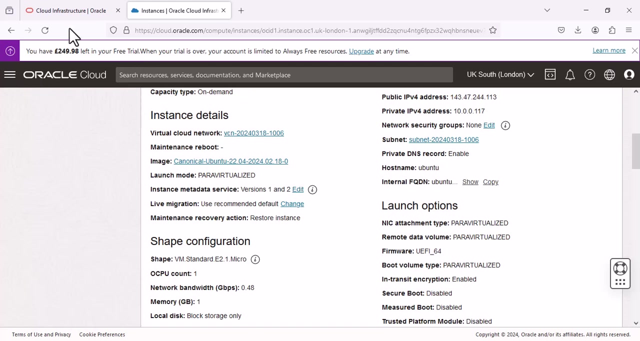 the well, well, uhh, well, you, which is ocpu, um, so you, if you are going to use more than that, what they are offering, then you have to pay for that simple. is that why they are giving you here 250 pound or 300? because once. 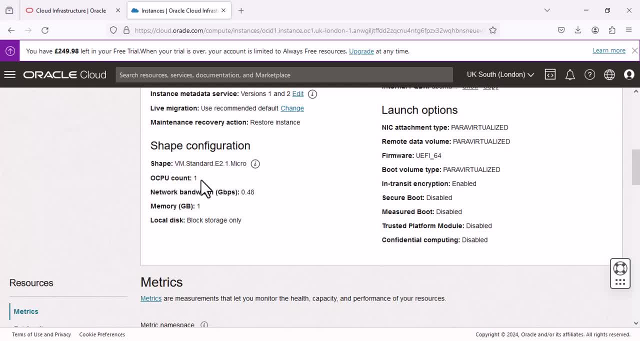 you will create, you will be using more than what they have given you, and then they will start charging you accordingly: how much you are using memory, how much you owe, or cpu, or cpu you are using, and bandwidth. so this is for this server. now we go back to another. 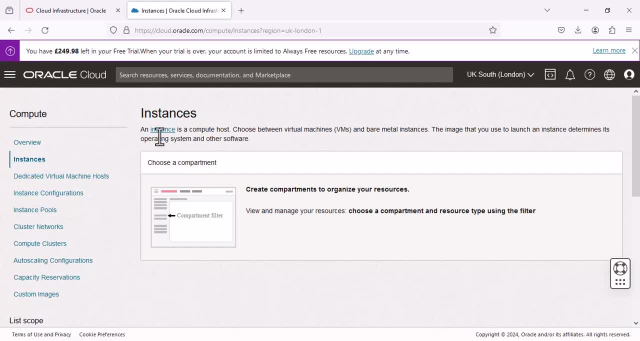 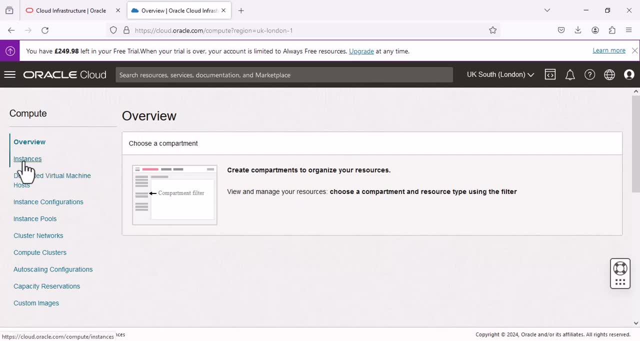 another instance, okay, compartment: okay, i'll show you what they are saying. the simple thing is, when you click here, they have- i mean they have to show the instances are running or installed, but you have to choose the compartment which is the typical language they are using, not for the beginners. i mean, then, what you need to do, i tell. 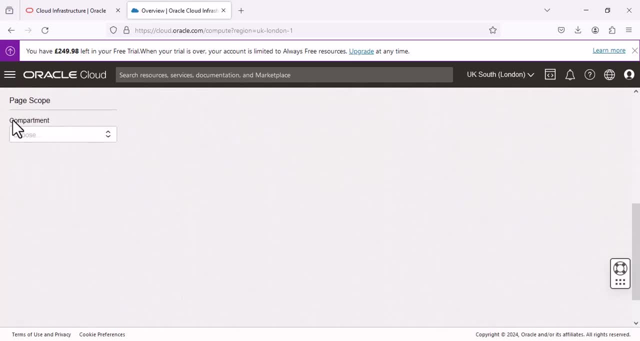 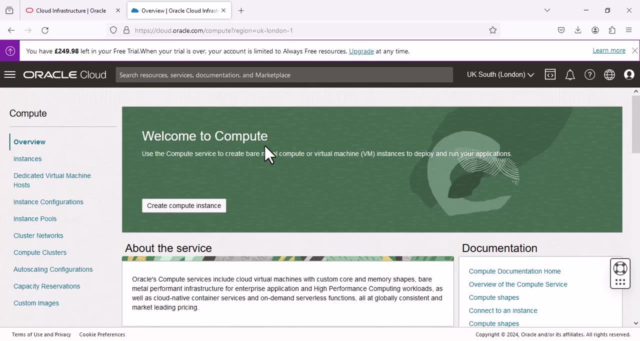 you simply go down- this is the compartment on your left hand side- choose the compartment which is your account- error 24 uk- and then click it and now you will see here either you can create um instance or you can just have a look your instances. so i've got two instances. 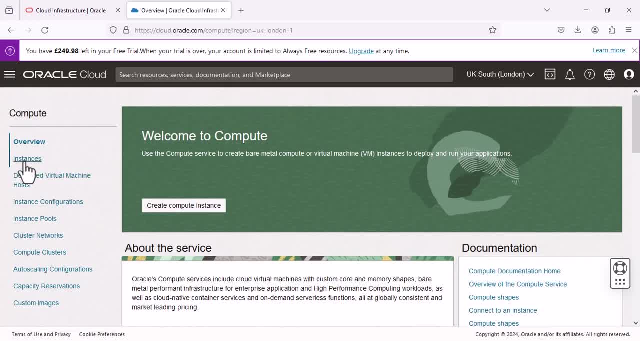 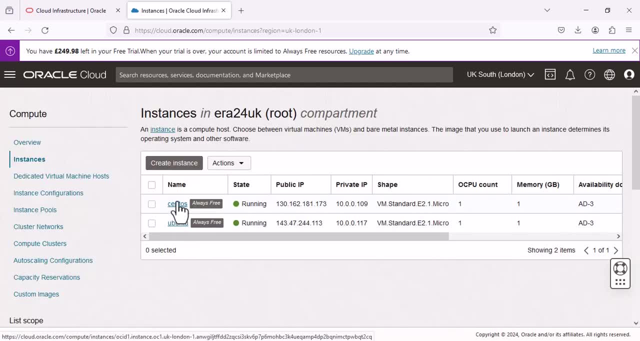 and now we go back to instances. so next one is centos, which is always freeze, written um, the same information you will find once, or cpu, one memory and availability of the, the, the server they will provide you, which is ad3 um i created on 18th of march 2024. 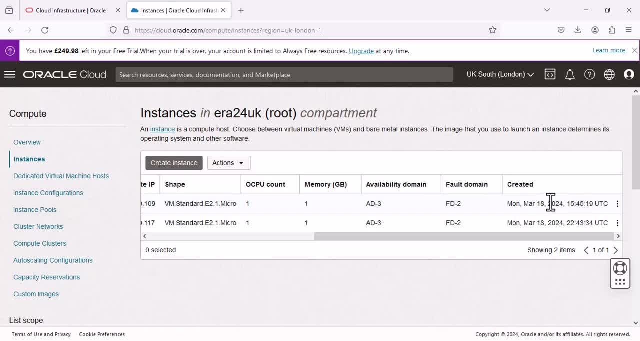 and today is 10th of april 2024, so in seven days anyway, the account will be limited to my sources, but i couldn't use them because the softwares i'm trying to install are. i'm unable to install them, and if i will be using the resources as 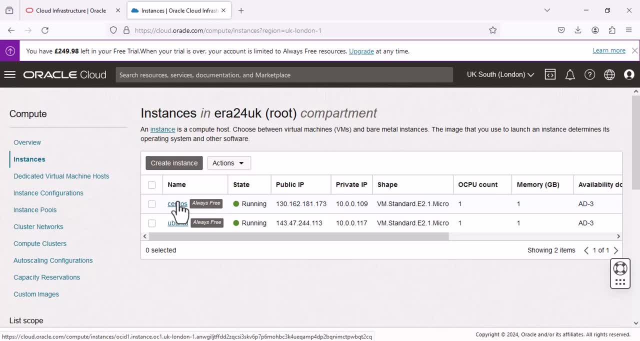 it should be, because use for your website and website platform could could be different. you can use php, you can mysql, you can use all other different kind of codings or scripts, but if you are going to use them on that, on their server obviously, then you have to pay for that. so whoever is saying that this? 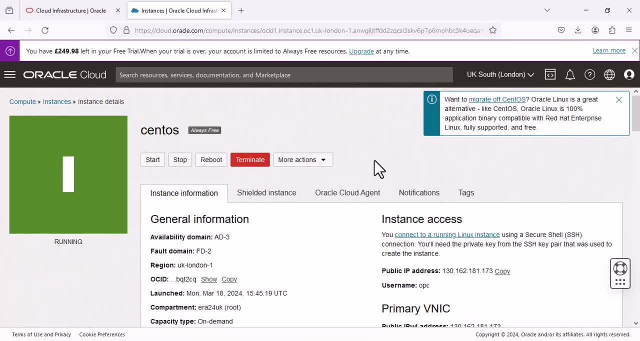 is free. i don't understand. please write me in comment section. if it is free, i will create and i will take your help to create. i'm going to show you what they are going to offer you. so centos, by chance i just installed because it was not available on any server they have. they were. 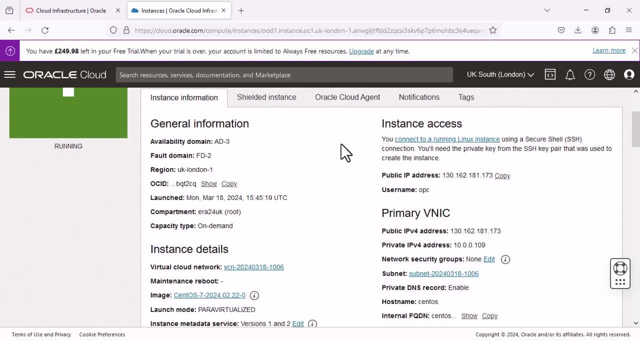 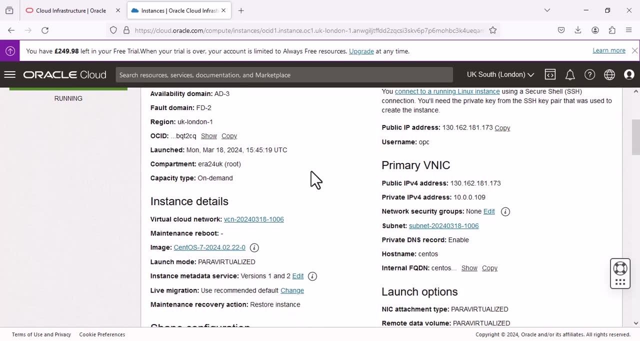 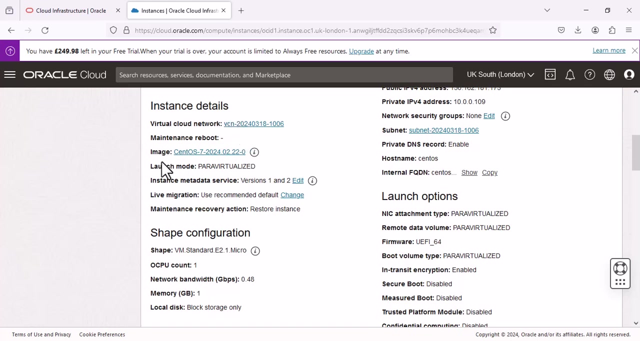 giving me three servers i will show you soon. so, first thing, we will go on centos and here you can see the same thing. the server name is ad3, the region as i am in the uk, so uk, london, one. um the other information, yes, i show you. this is the other information. 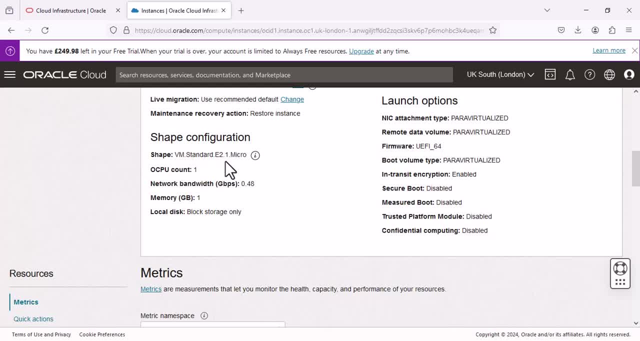 so i'm on shape shape. they have given me um vm standard e21 micro and this shape does not support resizing. you see, up, there is a message. this message is saying: this shape does not support resizing. you cannot. you cannot extend to to ocp or or your cpu to cpu. no, you cannot extend your um memory as well. let's see. 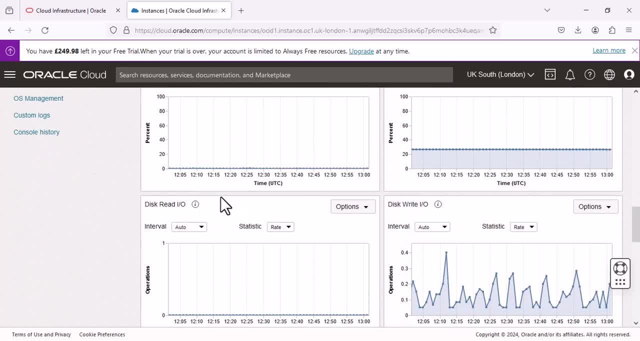 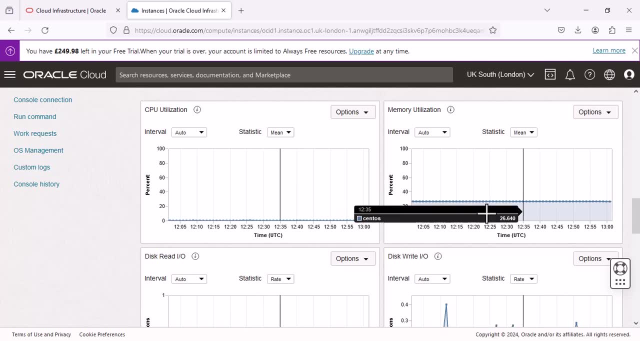 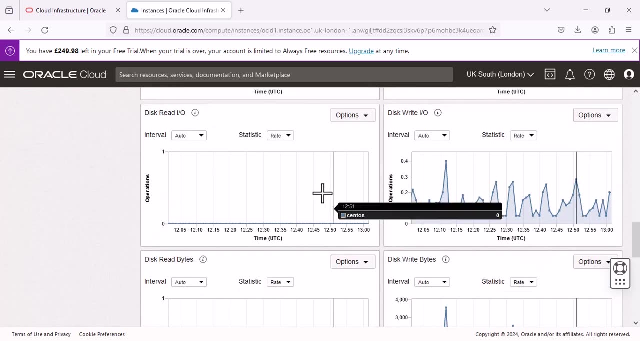 what we have done. here we can see that we didn't use um up a cpu utilization. nothing is used, same way like memory i didn't use. but it is showing that something is using um disk writing. i don't know why it is writing when i haven't done anything. 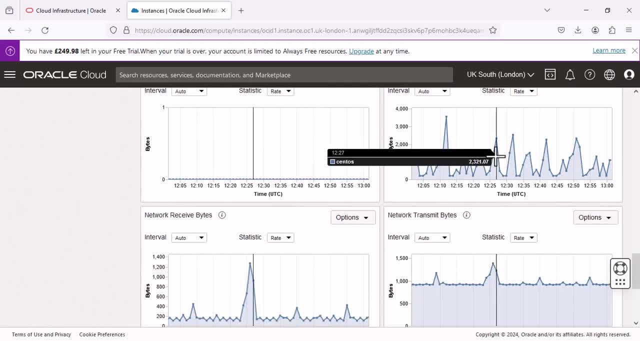 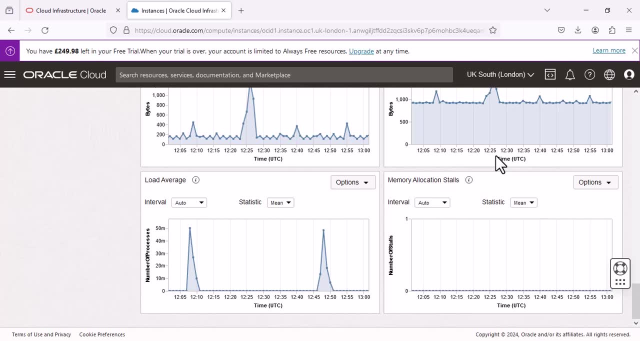 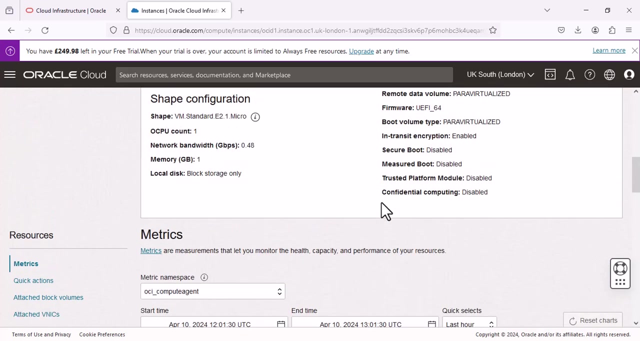 uh, not even access remotely, or maybe it is because it's just running. so this also will be counted as you are using the resources, and if you are beyond the limit, then you have to pay for that. so be ready and make ready your credit card or debit card. um, they, they will. 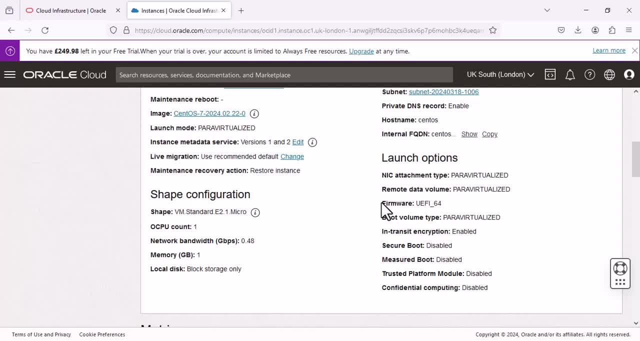 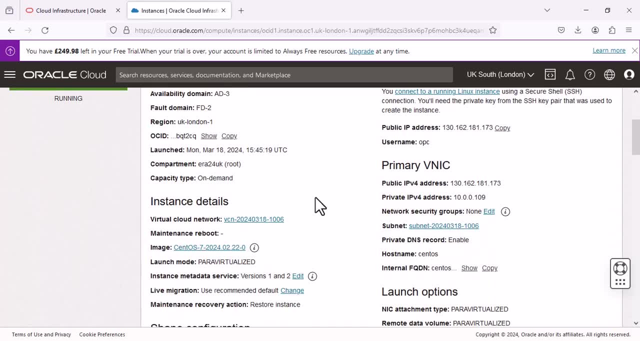 charge. they will charge you, as i showed you earlier that they have charged me a 2p. i don't know for what. i didn't even use that. oh yeah, i didn't even use their servers. but there is a small charge, i don't know for what. 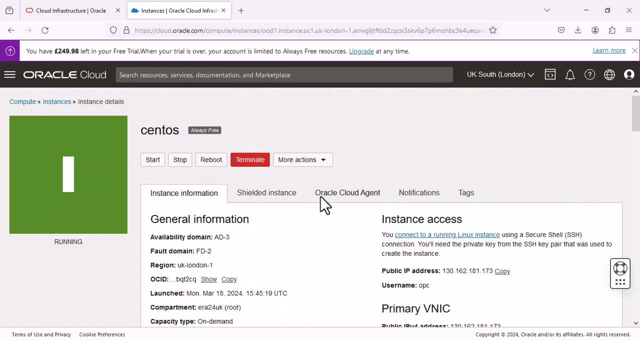 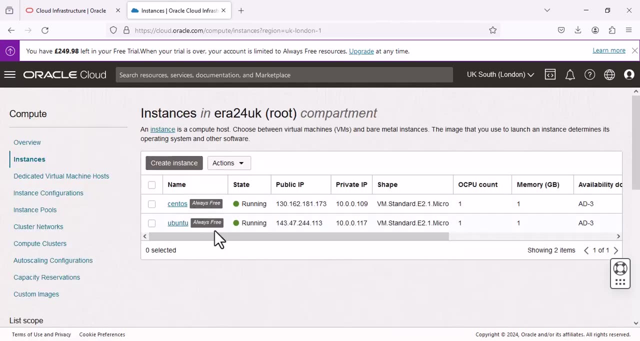 but there is. so be ready and make sure that you have good enough money um to invest and get these servers, which is which is called free, always free. they are not free, they are. if they are free. yeah, you can see what they are giving you in free: one cpu, one pc and one mpc. 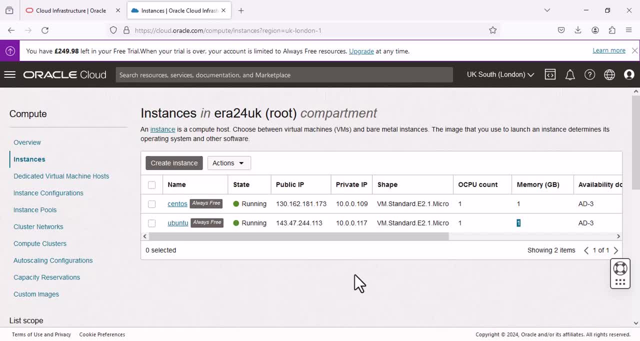 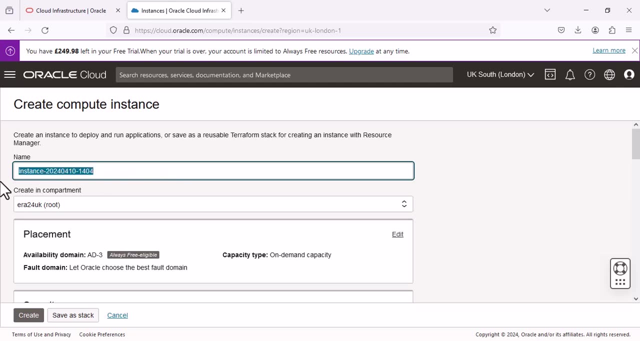 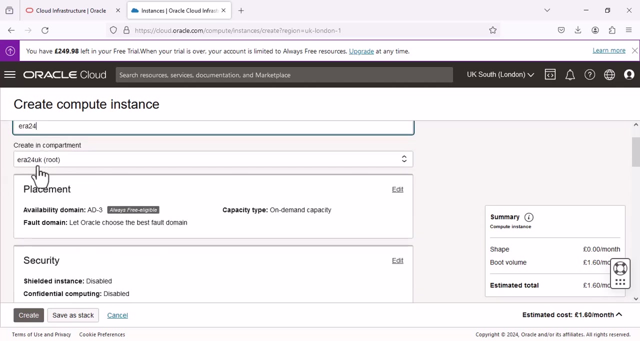 memory, so i don't know what you will be able to run on these kind of servers and to create a new server and this server name i'm going to give you um era 24, just for the sake of video. so you see, i wrote, i just inserted the name of the instance, the compartment i showed you you can. 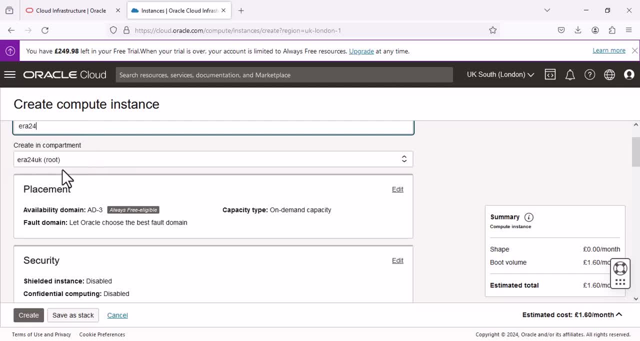 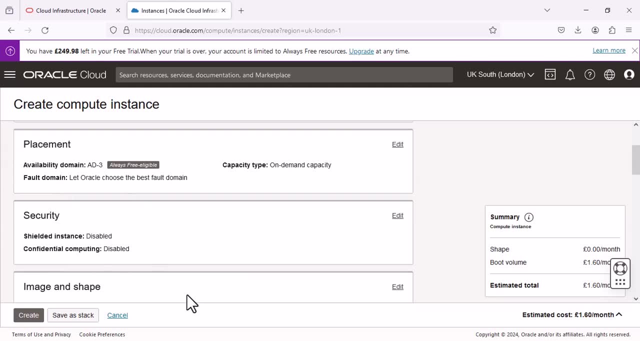 choose the, which is the root one on the left hand side, and then now they are giving um two things: on the left they are giving you offer and then on the right they are giving the price. so estimate: cost: one pound 60 pence per month. per month you have to pay. okay, still, i didn't set it up here. it is saying always free. 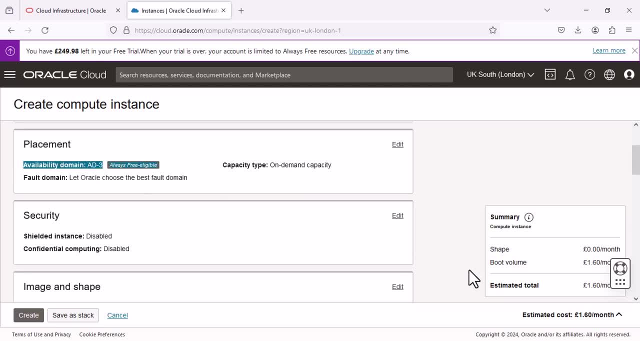 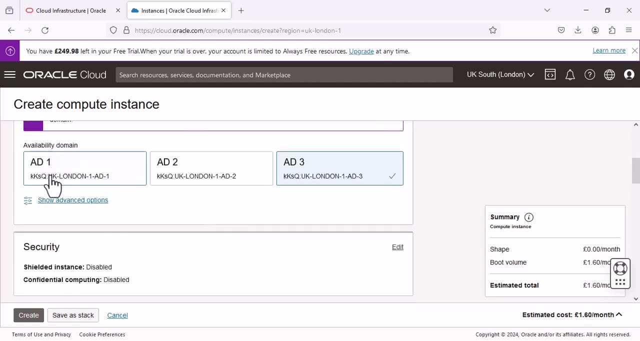 always free. it is not always free. when i have to pay one pound and 60 pence per month, it is not free. so if you add, if you say okay, i'm paying and i need to check um another server, um, maybe i will check with this server um which is ad1. 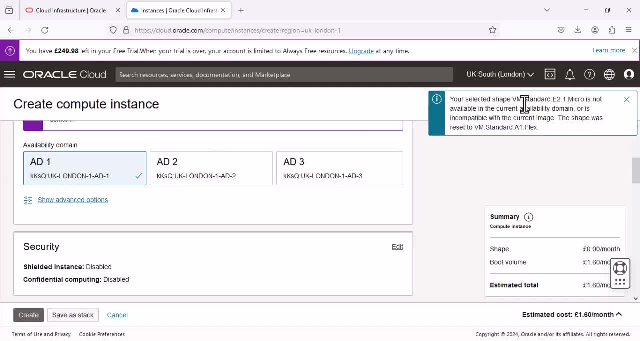 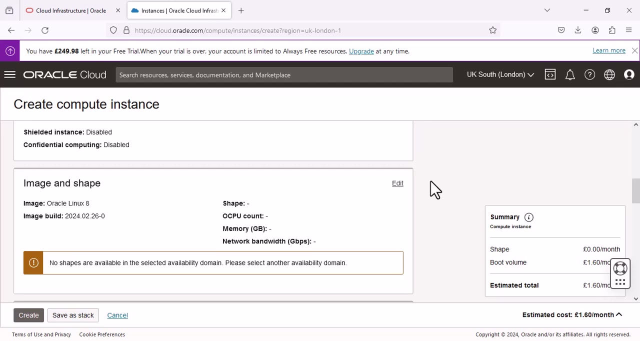 now this is saying your selected shape vm standard e21 micro is not available in the current availability domain. if second one also showing an error, you will see on ah. so oracle linux 8, i don't need oracle linux 8, i need, i need ubuntu. i need um others, other software, debian- okay, i let's. 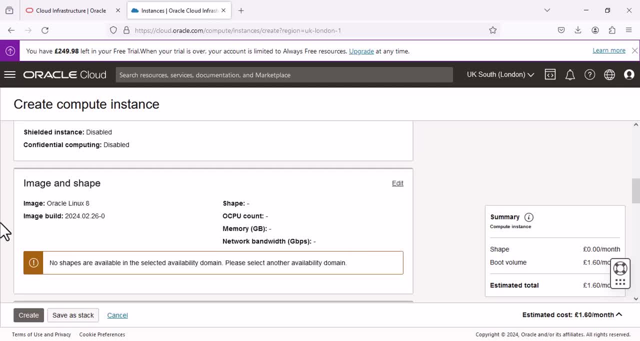 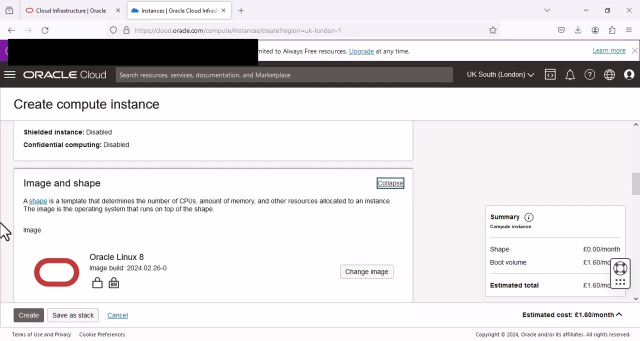 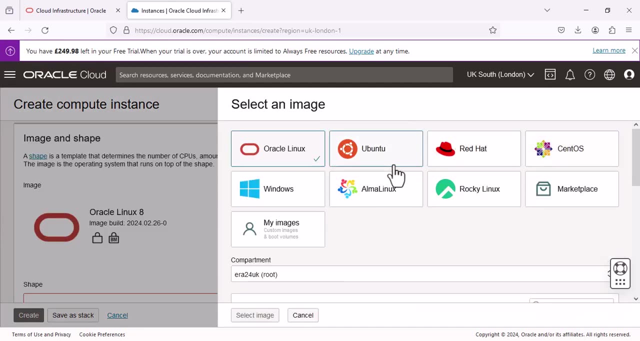 change the image. now they have got um ubuntu, red hat, santos, for example. i'm just going for santos. so and, and once it is selected, let's see, i cannot. i cannot select image. i don't know why i can't select image. okay, i will scroll down. okay, so, after scrolling down, they are asking which? 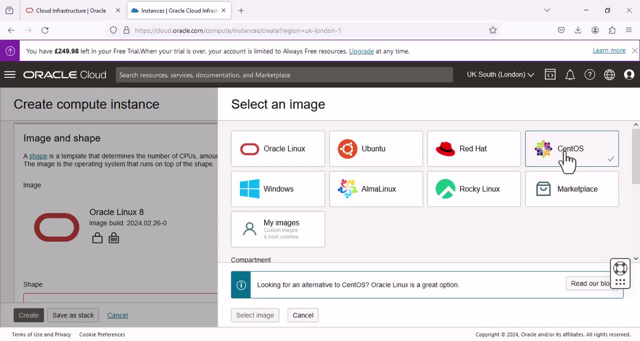 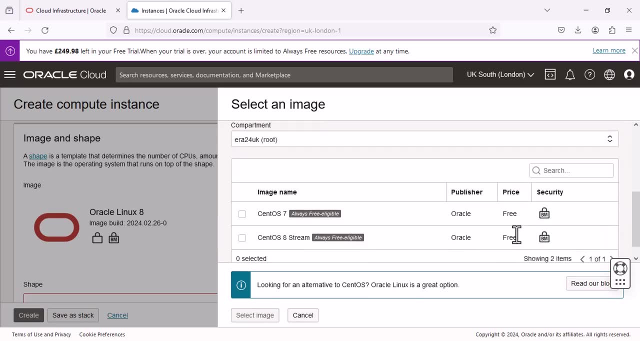 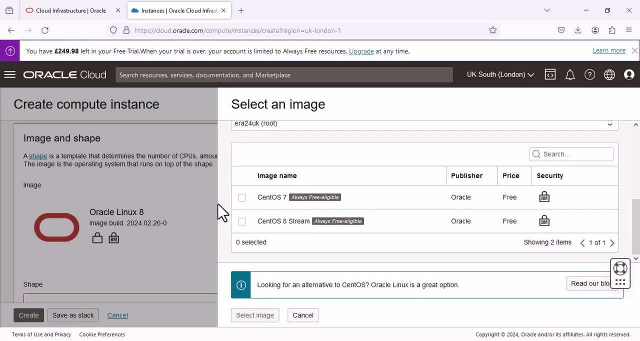 operating system and let's see if it allows. okay, you see, there is a message: shape: you chose operating system or you choose operating system. they don't allow you, so they only allow whatever. whatever is rubbish, i mean, it's not in your use, as i said earlier, you 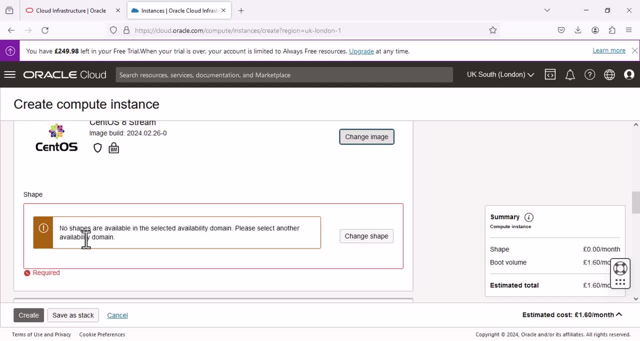 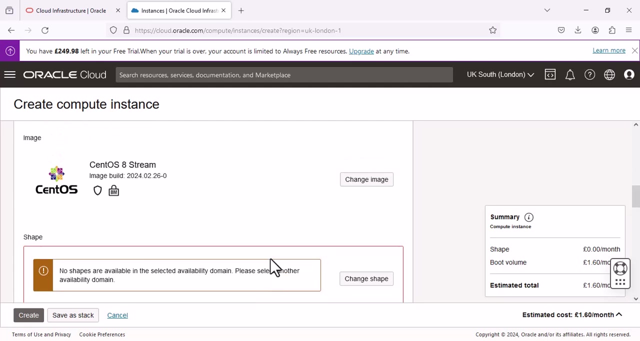 can use it for your practicing, when you are, while you are learning and and experimenting. yeah, then you can create any um, linux, os, and then they will provide either shape. now i don't have a shape, and now you will be thinking: what is shape? actually, shape is your uh server, which is uh, depending on how much ram, how much. 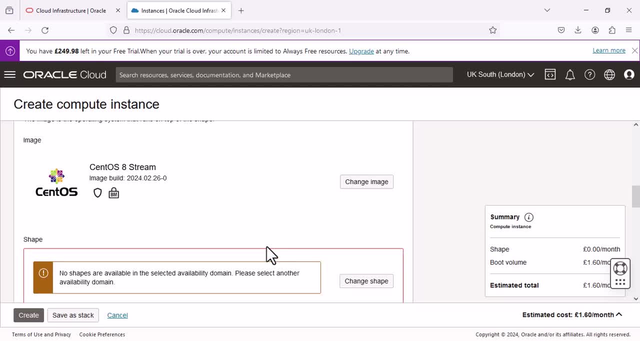 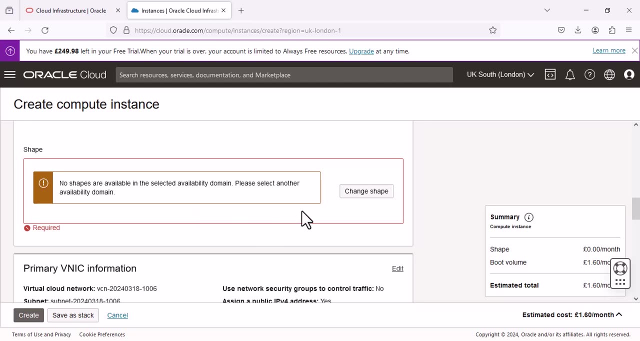 memory you are going to use and what bandwidth you are going to use and what operating system you will be able to- i mean able to use- but as they have already given you, you will not be able to use on this server this operating system, which is santos 8 stream. now we change, for example, 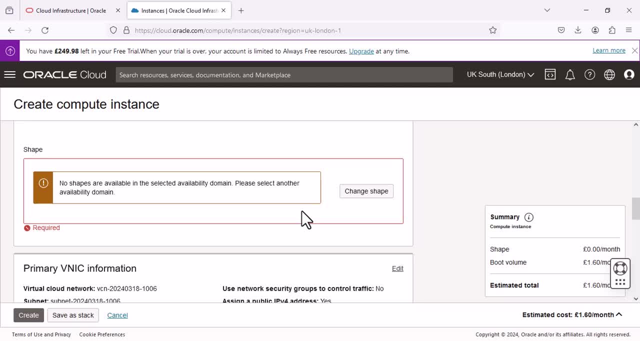 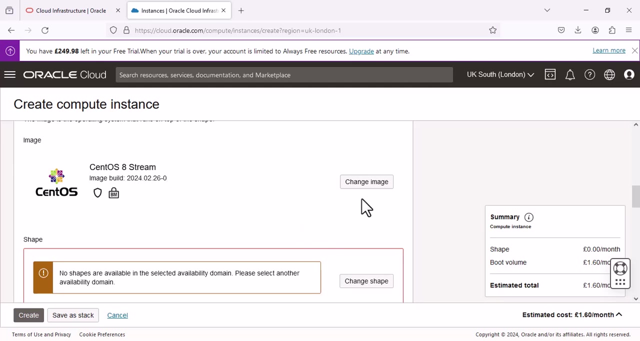 and try to take ubuntu, and in ubuntu as well, same thing. they are asking which version? okay, we are going to choose the latest version, so i will choose this and click. you see, this one is also not available. okay, let's try the, let's try ubuntu. and the minimal, the small version of. 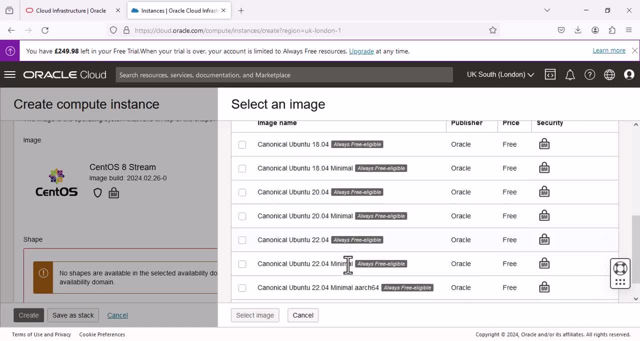 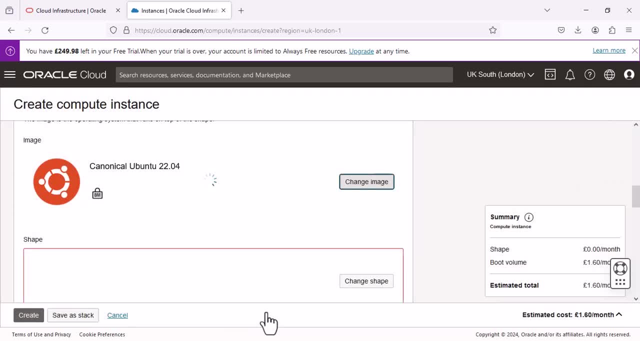 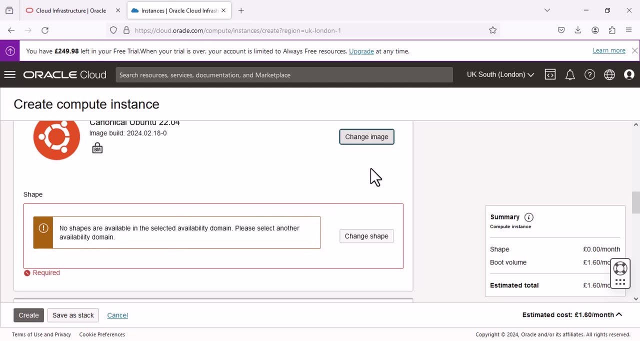 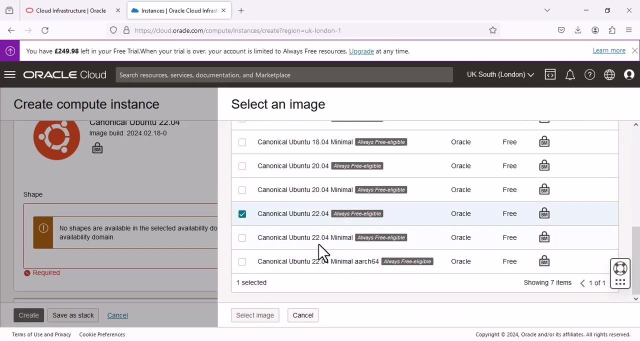 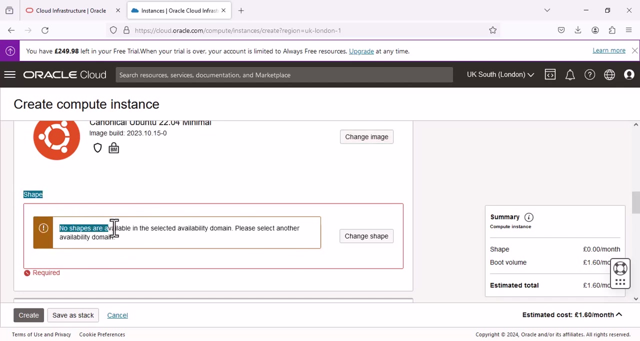 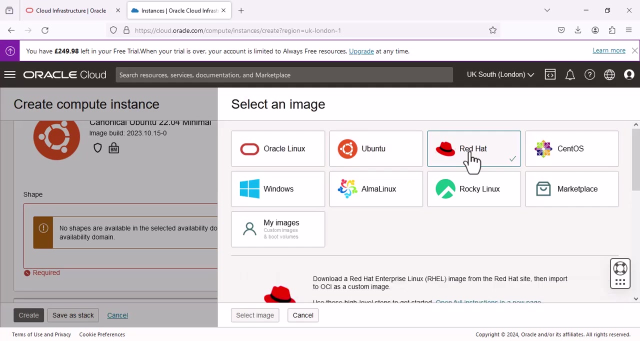 small version which is free. select small version also. you cannot install. so what you can install, let's try another one. maybe i just go and try red hat, red hat, okay, red hat. oh, you have to download red hat, enterprise um linux and then import to oci. okay, so you have to download this thing and on your system and then 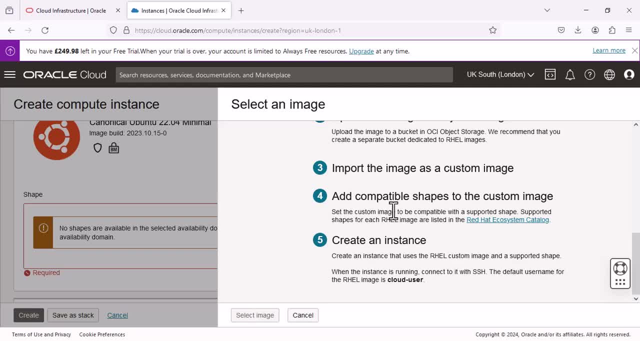 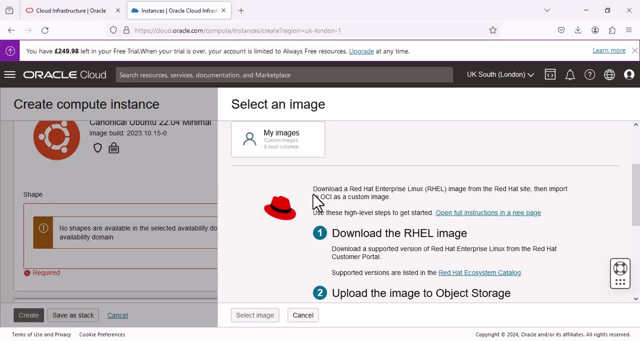 upload again. uh, let's go to windows server page and quickly go. screen telled: uh, you know you have to download theわjd. ok, i've done already. then click to install window. which windows server is it welcome? oh, oh, another headache. okay, so i don't install this one. i just try to go and install windows. i. 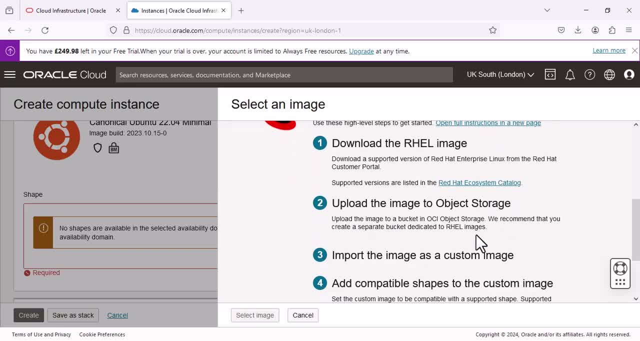 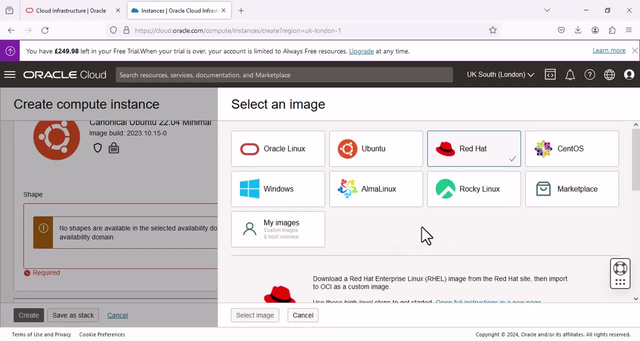 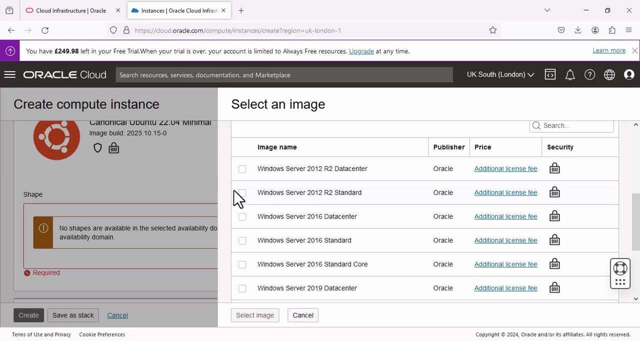 install windows. i ask windows server, which windows server? i will use um and accept the following document. so you have to follow this document before you are going to install windows server on. if they will allow, let's see what's come. okay, so they are giving you nothing different, nothing different. price is straight away coming up, but but whatever you 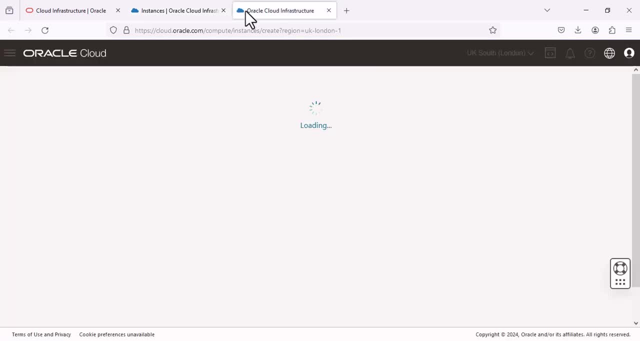 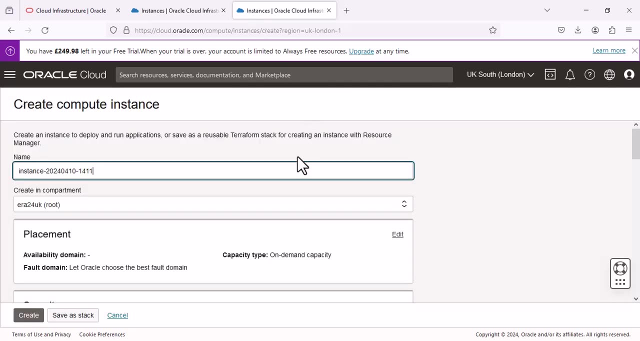 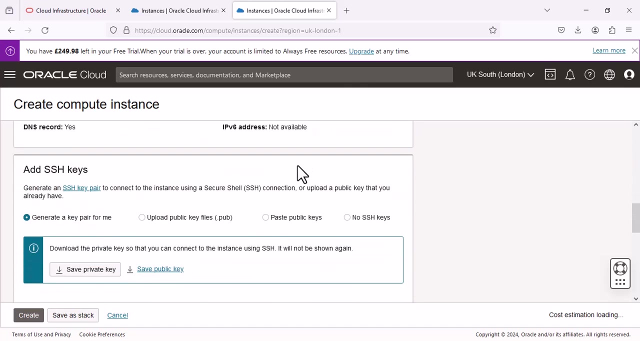 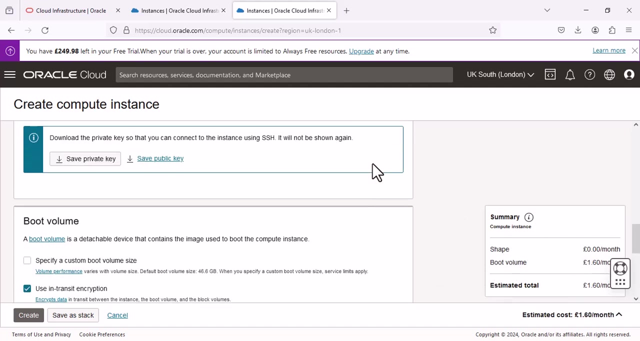 need to use. this is whatever left over. you're not left over once. you don't want to have it and then give someone. so this is the, this is what you can have it, but not for your um, for your websites, wordpress website, for your server, for you know, storage manager. 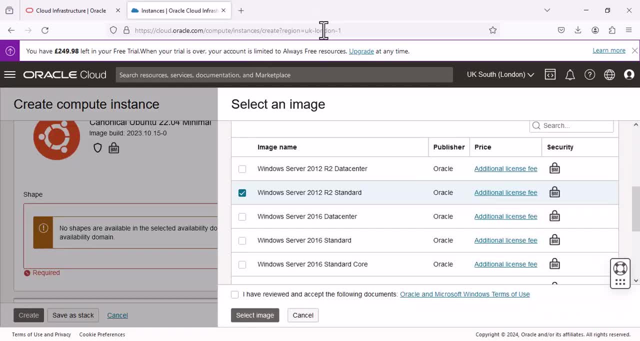 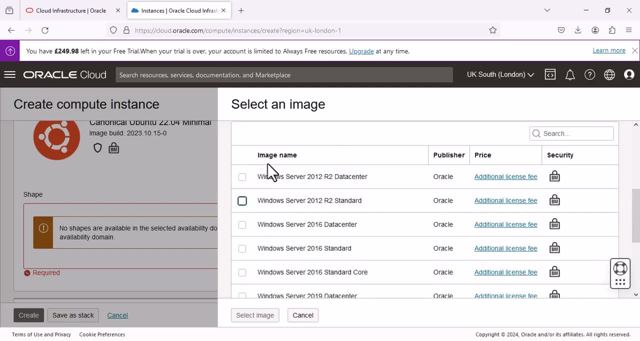 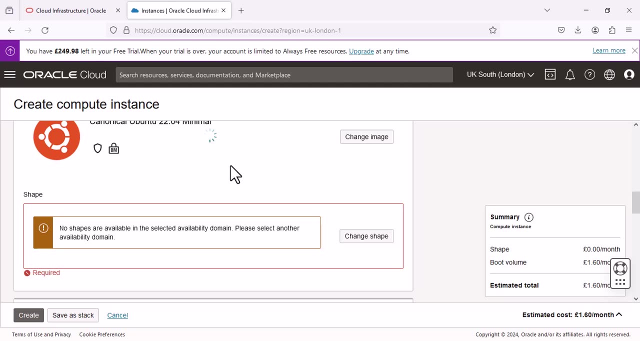 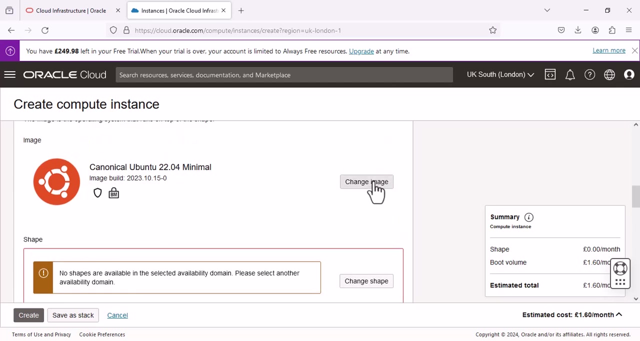 download. you cannot use it. okay. um redhead, i showed you os. i showed you i mean centos. i showed you. um ubuntu, i showed you windows. i showed you. uh, this is the alma linux. if you want to install. i don't know they will be able to accept the installation. okay, i just. 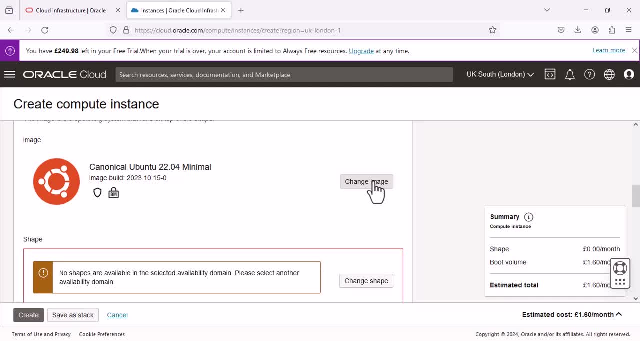 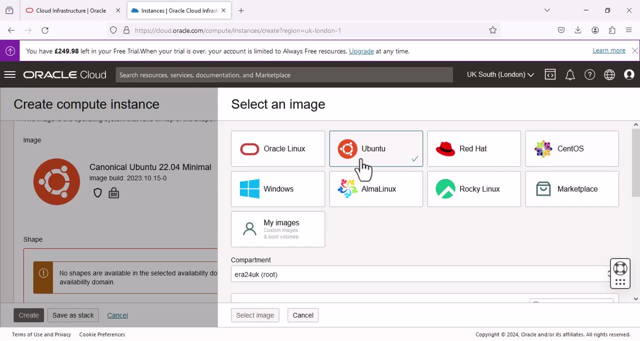 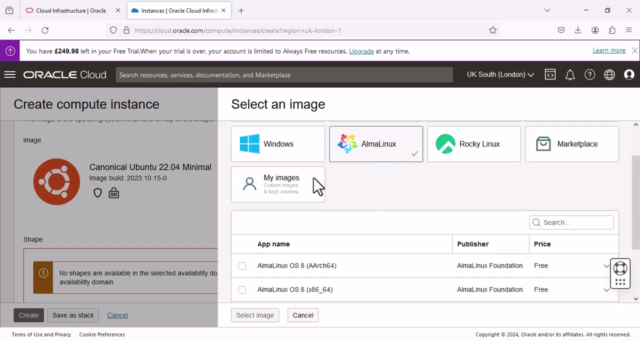 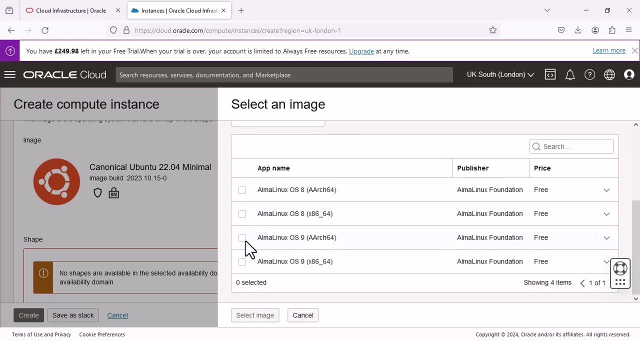 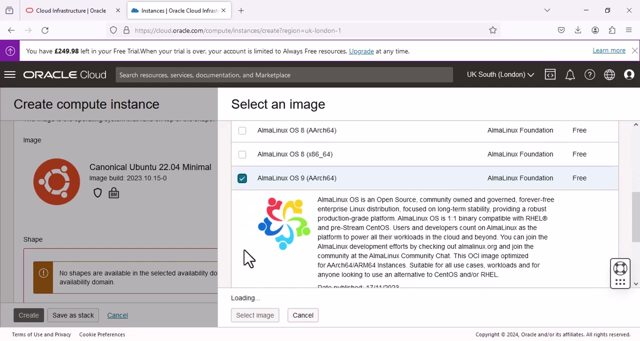 choose the alma linux and an alma linux. you need to choose, for example, 64-bit okay software. and here is also an agreement. you just need to read the agreement terms and conditions, partner terms and conditions, oracle, general privacy or privacy policy. once you select this, then you collect and it's also not available, so the shapes are not available, which is server is. 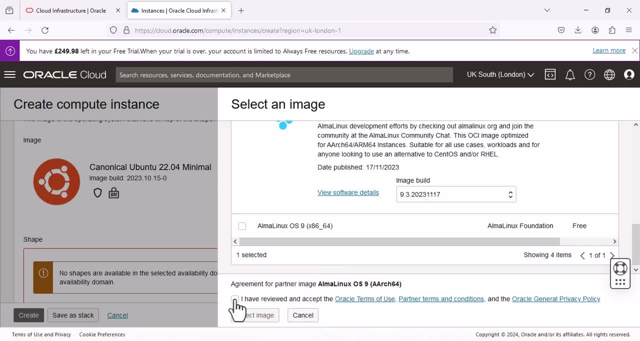 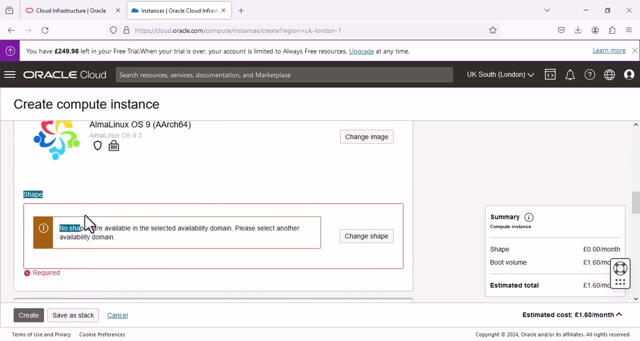 not available when operating system is available. so if you like, you can go for oracle cloud. i think i did a big mistake. it was a wrong choice. i just wasted my whole month for nothing on uk south london. this was the location, or or the region, because other regions i cannot choose. 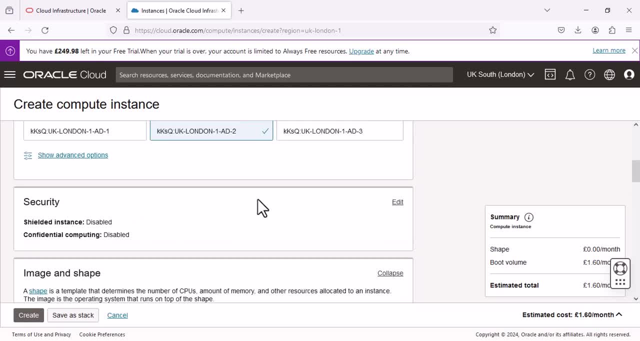 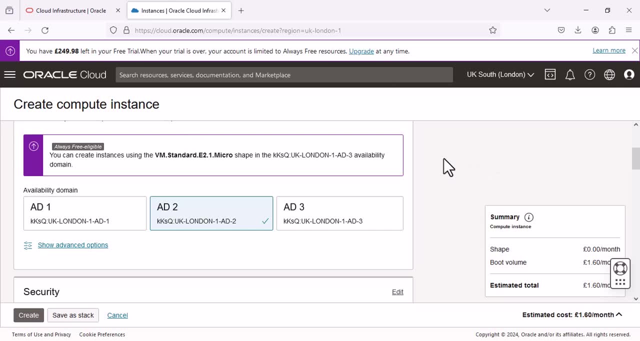 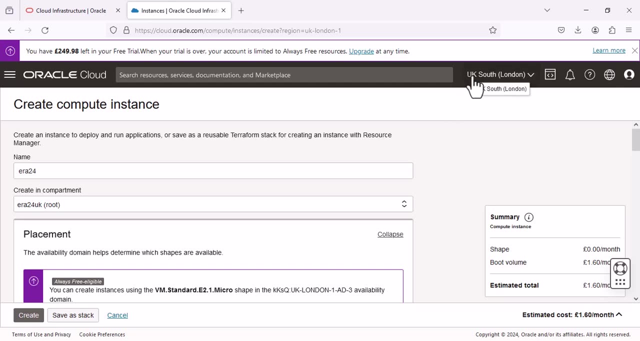 if i go and say, okay, i need manage my region and here. if i say, okay, i signed up for london and now i just change to, because right now i just i didn't. or if i created a couple of servers or instances, i can, i can delete them because i'm 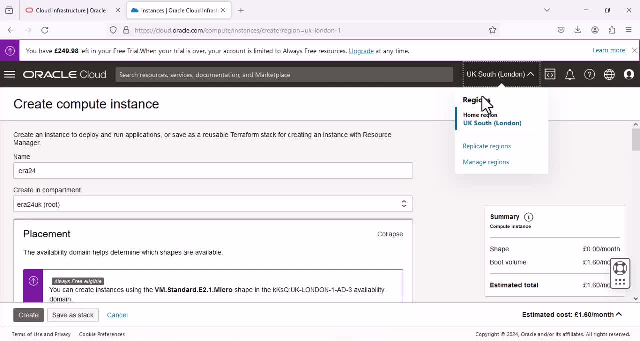 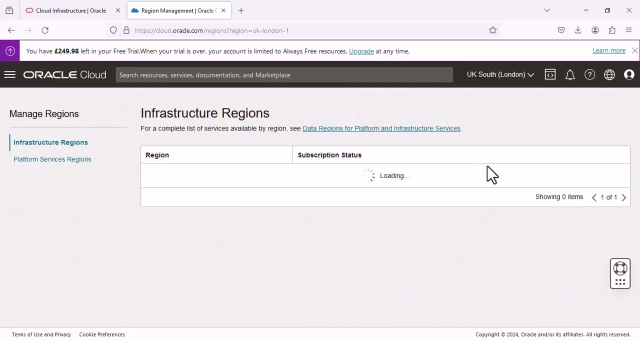 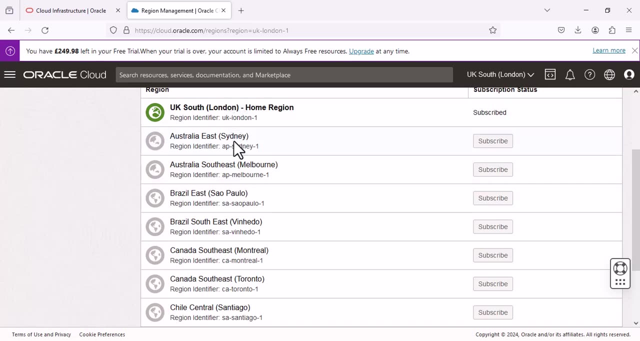 not using them anyway. so if there is any possibility to change, i would go, maybe any other country, for example. i just show you if i click here and here it's nothing happening. nothing happening with the any one of them because you you see this answer of their. 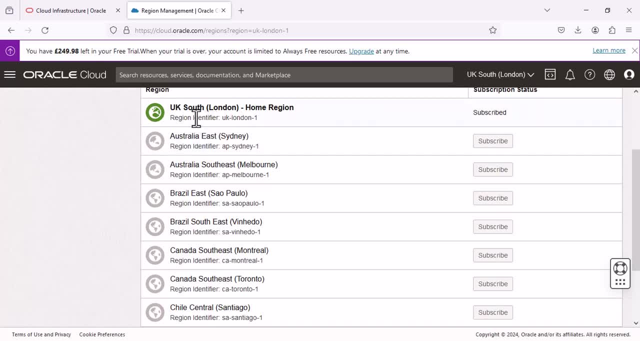 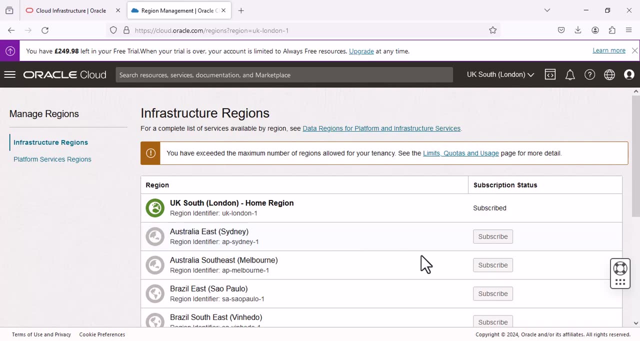 question or our question. you have exceeded the maximum number of region allowed to your tendency. okay, you are giving us free one, so obviously we can have it one, but allow us to choose any other one. we are not going to take all regions and we are not going to take all regions. 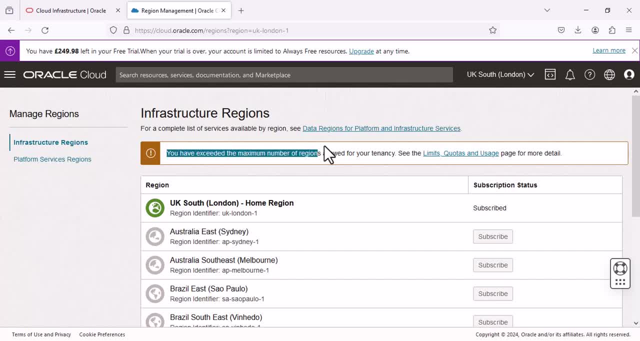 or we are not saying that in a month time, in a week time or in a two months time, three months time? i have changed so many regions that you don't allow me. this is the first time. they have to give us a little bit flexibility that we can choose which server region we want to choose which one. 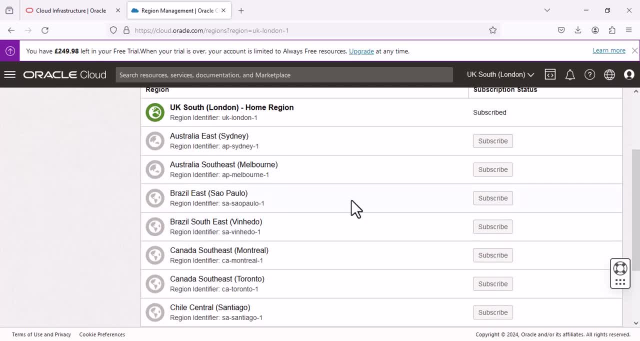 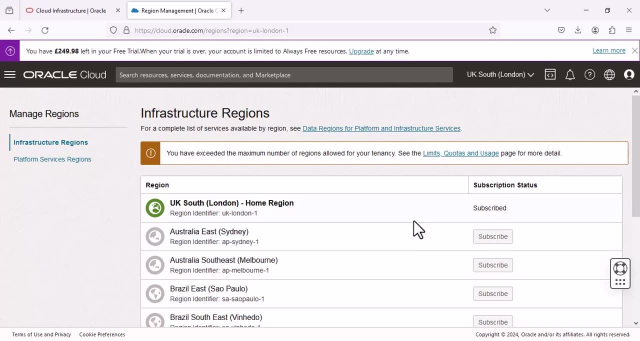 is better for us. no, no, no, you cannot choose it. whatever you have signed up, you will stay with this one or you closed your account with this one. you cannot choose any other subscription, so this is a very bad thing. i cannot go anywhere else if i chose this one. so this is the one, and you have seen uk. 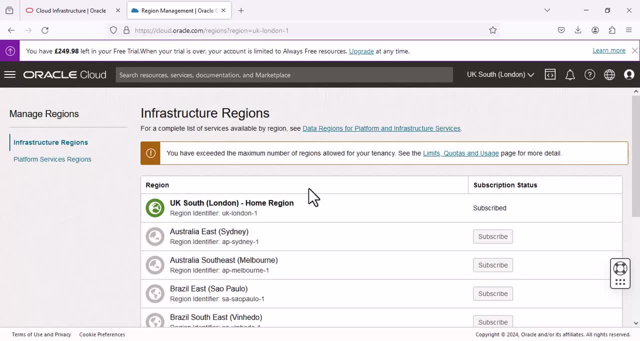 south london they are offering rubbish servers. i will not go for that, so i'm going to close the account. but i am going to close the account in my new london system, just like that, is it? yes, so that's the first thing that i was doing now, while i'm recording and ex explaining you the the situation. 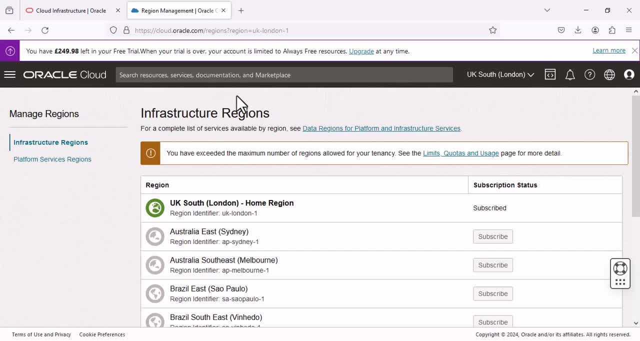 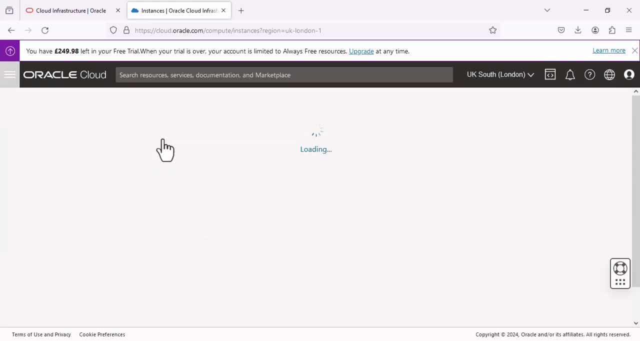 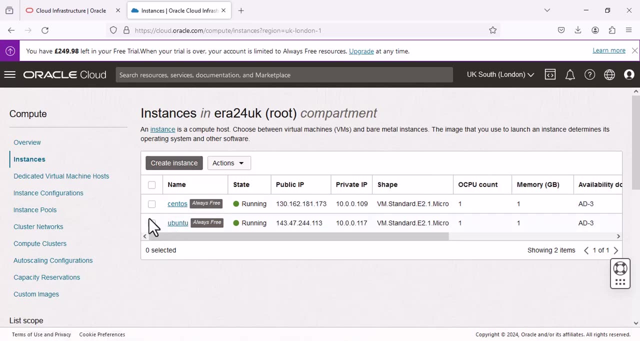 because, um, it's useless. the centos is there, but the thing is, the memory is one gb. in 2024. who is using 1gb servers? can you explain me who is using? um not taking too much, but the thing is, you are going to install on on these kind of. 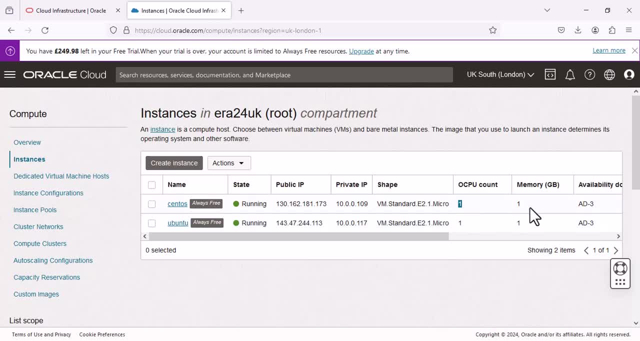 operations systems. you are going to use other software's. the other software's will be running a server, a server running. we will be running your website. your website will be taking space, storage, memory and bandwidth. so one memory- 1gb, memory 1gb or CPU- and then they will start charging you. so this is 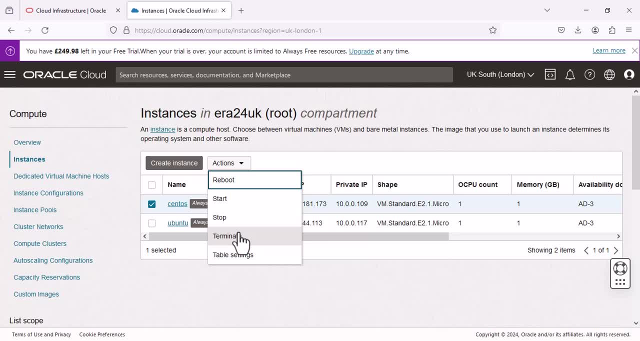 a hidden kind of you know, I don't. I think this is a another business. okay, I'm going to terminate. so I just check this one. I went to action and from action terminate, so permanently delete. yes, I want to delete permanently. okay, this one and terminate. now it is terminating the server because useless. 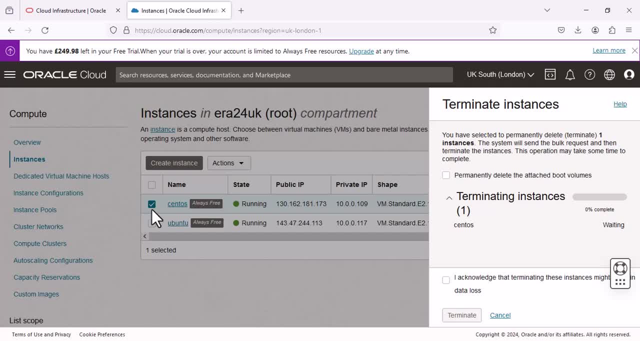 for me. I was thinking they will be giving 4gb RAM, 16gb of processor or or like here they said I don't know, maybe 16gb memory, 4gb or CPU, and I'll just fake this and save this, but it is a 100 gb RAM, so I am going to. 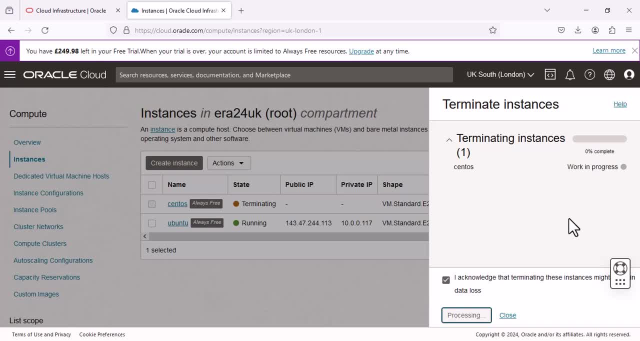 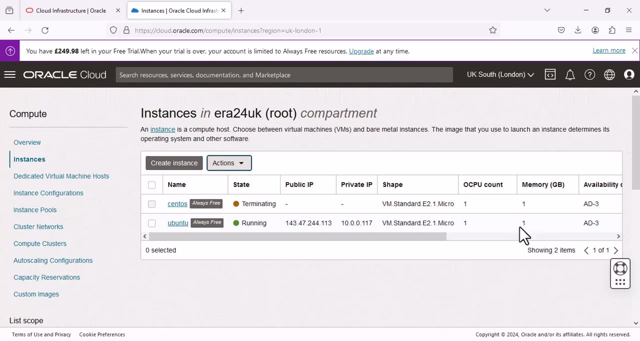 terminate them now. let's check it, but they've already let me finish the server. but you can do that. you can change the server name and also caramel server. so I'm going to change the server, but mostly I'm going to change the server name. so I'm just going to change the way they want this server name to be. 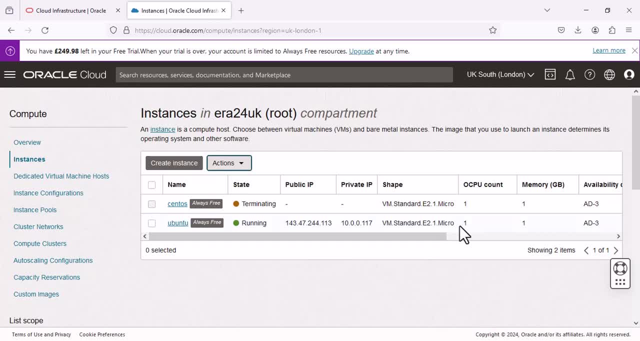 later. so let's see how this is going to work. okay, let's see how this is going to work. okay, let's see how this is going to work. okay, to terminate, front of you, I'm knitting permanently. delete, okay, and it's also in. 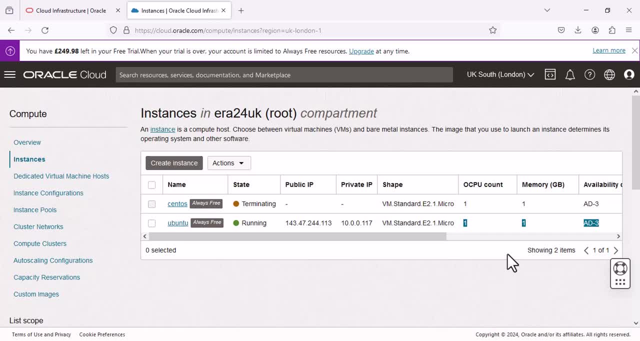 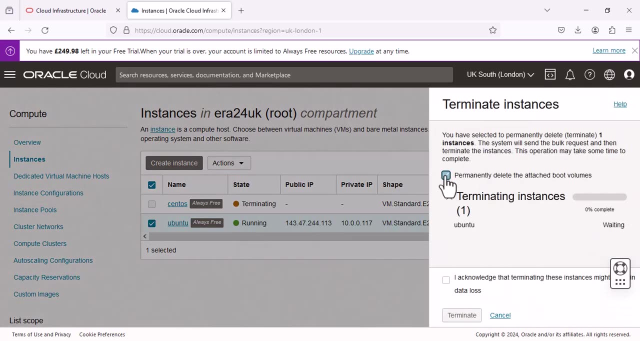 progress, the reason why I created this video, because everyone is showing you the golden side. oh, you will go there. you will get a free tier of Oracle cloud and you will be able to adjust your memory and OC or CPU, which is CPU. okay, so you will be using 4 or 16 CPU and then 4 or 4 memory, 4gb memory or or just. 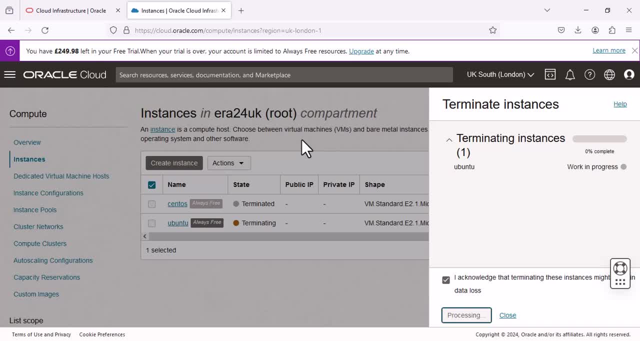 reversely like 4 or c4 or CPU and memory 16gb. but but did you see anyway, because I just tried to create an instance front of you, I didn't see even a shape of instance, because once I select operating system, there is nothing. this looks like they are making. 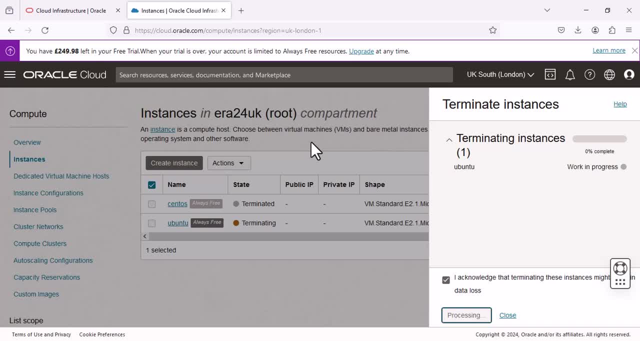 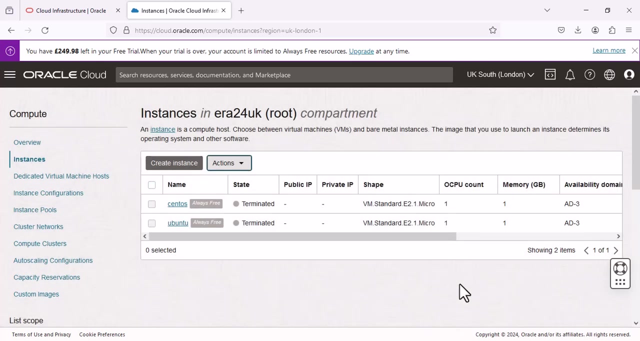 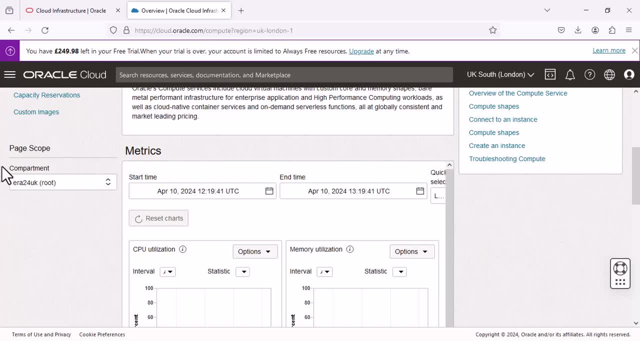 just write or click here and then choose this one. so this is your compartment matrix. yeah, you, you can check matrix. well, once your server is up and running and your websites are showing you the results I mean, otherwise I don't see any sense. see what they were talking about there. maybe they don't have any kind of you. 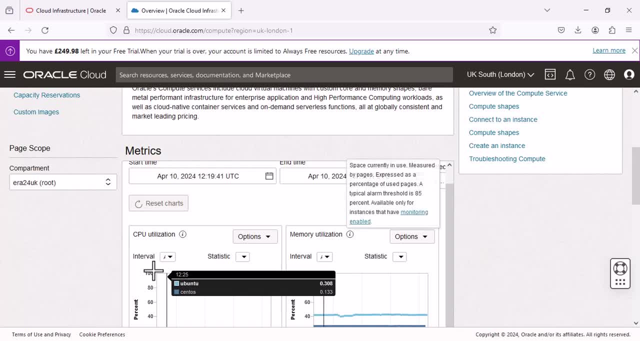 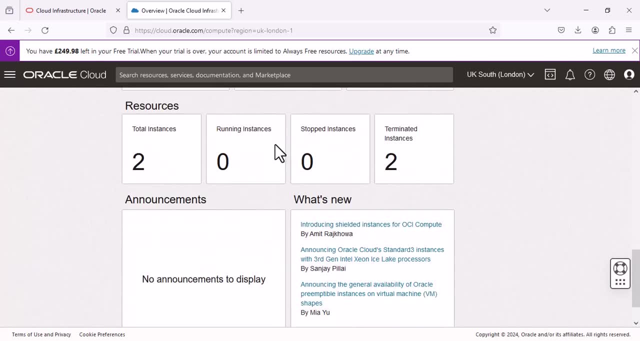 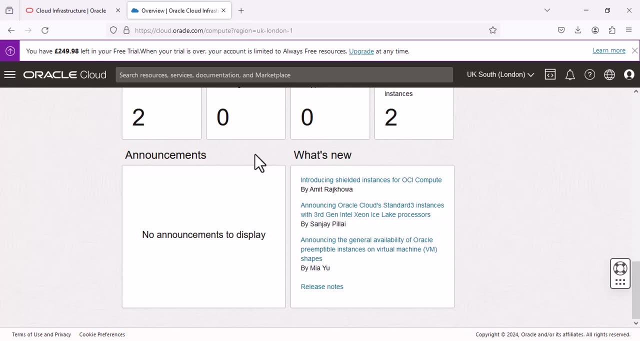 know like they can teach you something or say you something. okay, if you are using free, how will you be able to use free and how will you be able to increase this? there is no video, no tutorial, no guide. yeah, maybe the guide is in the PDF form or I don't know. like these kind of you know people are giving you some information, maybe you will find there a duck omega guide recipe. 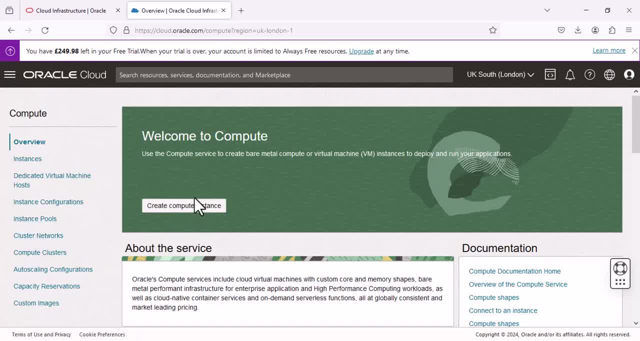 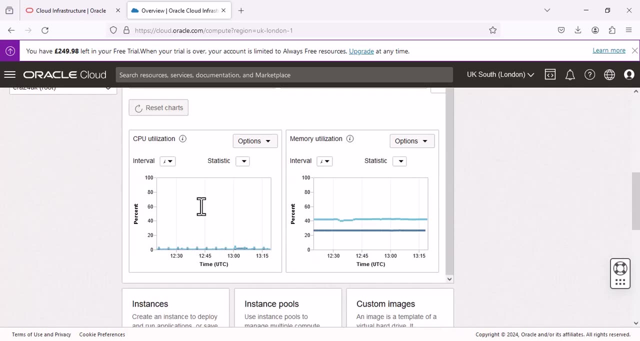 videos sometimes very sencill: Кıma тебе не нужно книг, Берете пров. futures video. Andrea the morningDavidWin documentation, like here, like, if i say, um overview of the compute service. so now you what you need to do now. you need to go through with this whole document, read and understand and then start. 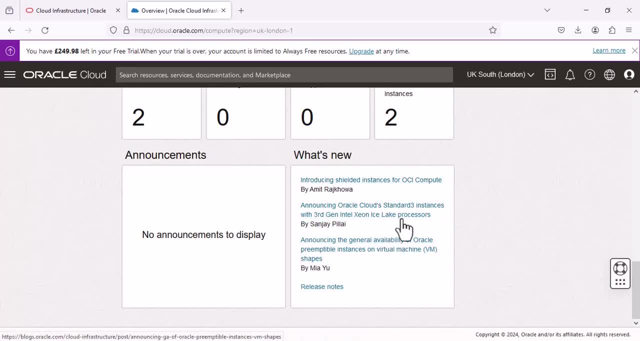 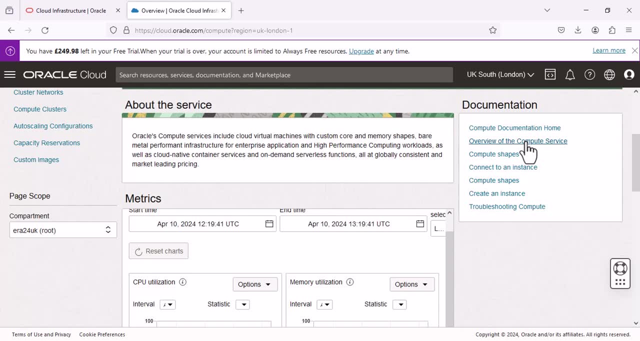 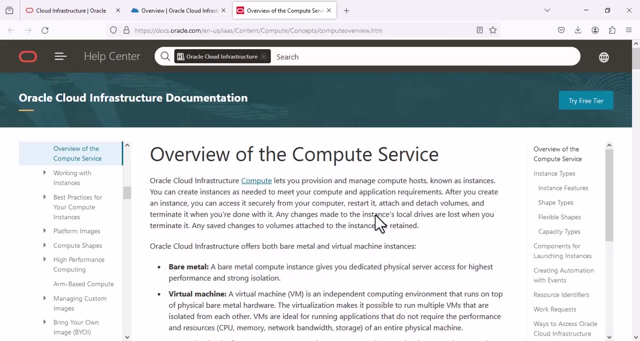 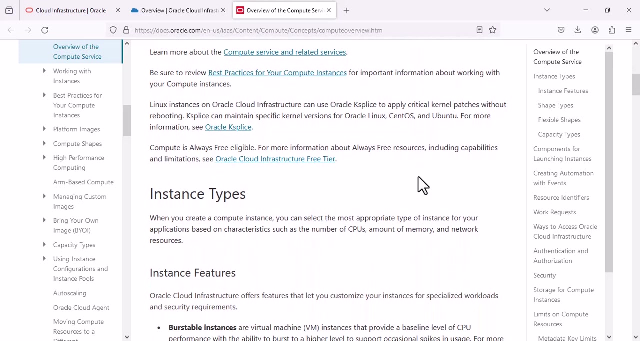 creating a single piece of instance, which is i showed you in a couple of minutes. it was so easy: just to click instance, go and choose your operating system and set it up, your server with ocpu and ram. but if, but if, if the shape is available. so if there is, shape is not available. 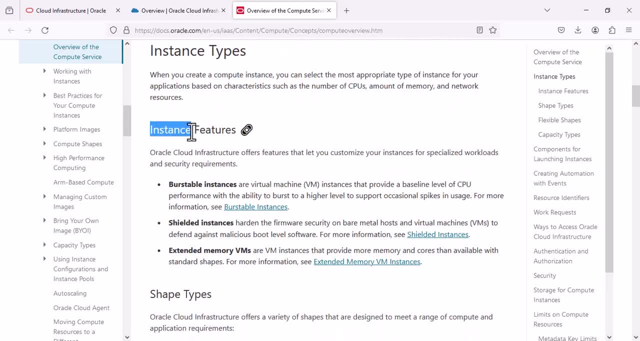 then whatever hosting servers you choose, um is useless. it's just waste of time. so write me about your experiences. maybe you have got signed up oracle and then give me where you were uh located and your servers or origin. maybe your service, the server's origin, is giving more and 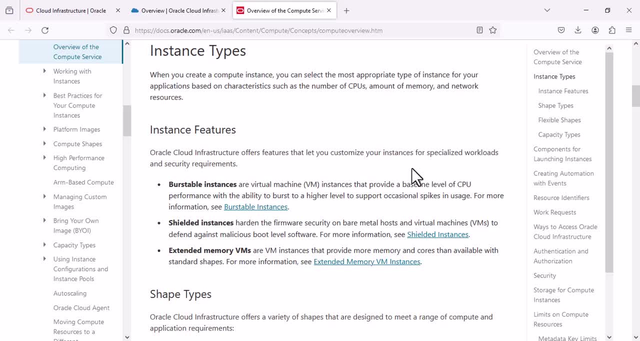 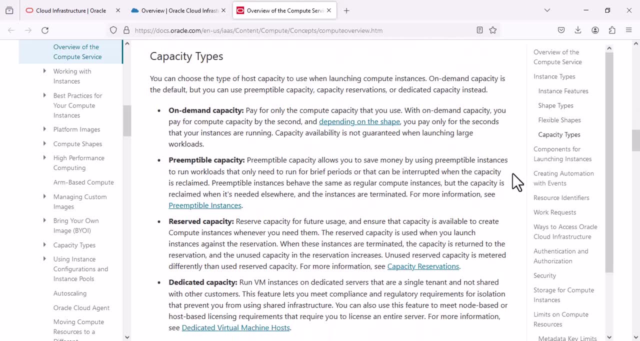 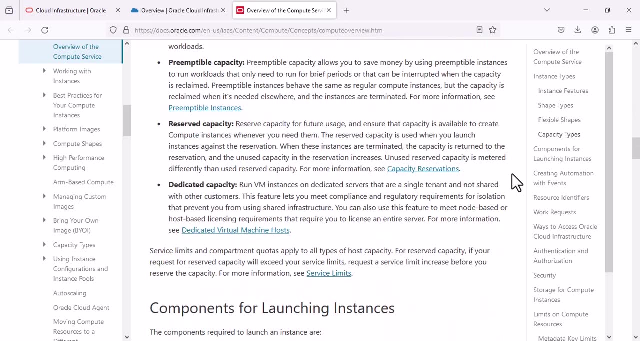 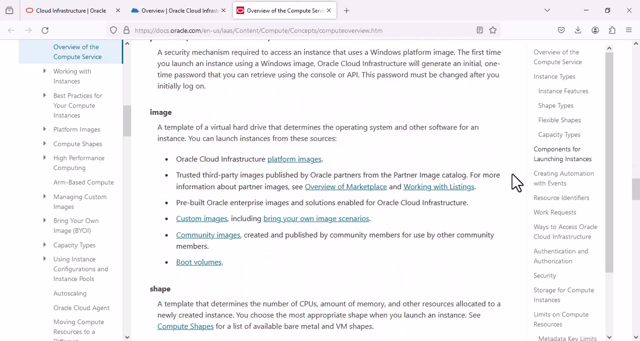 much better than what i have experienced- um, i have, or i had, because i'm going to close today. so i had a very bad experience because i'm not used to with play around with one cpu and one gp of ram. yeah, if you, if you are beginner, yeah, it's good for you, you go ahead, go ahead, use it. so it is good that you can. 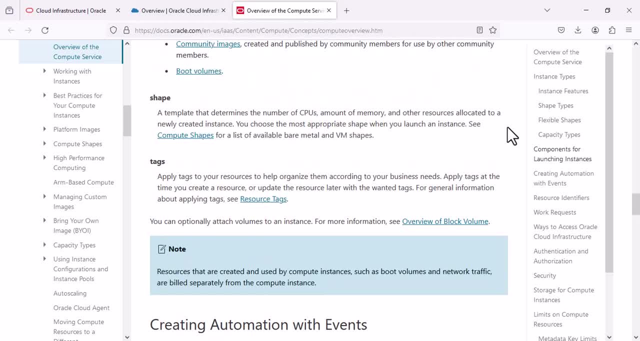 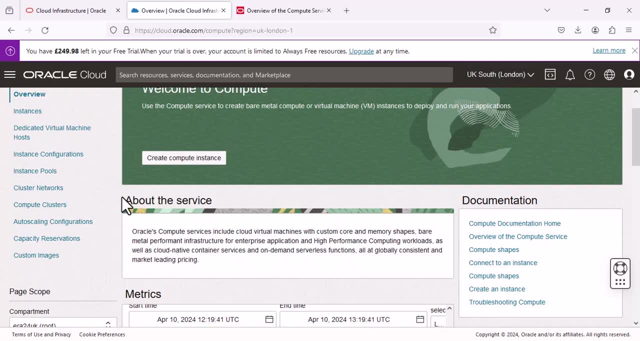 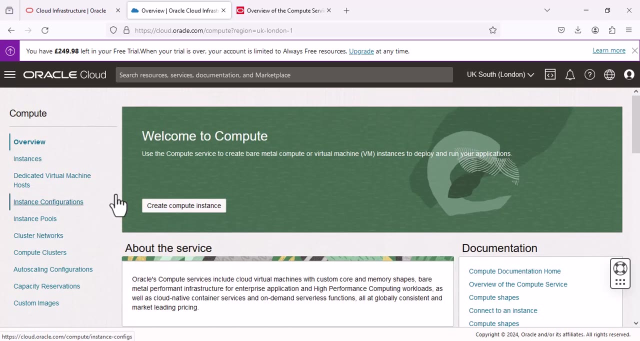 do some experiments and don't do some experiments beyond the the higher usage, otherwise you will be charged. so i'm going to close today's video and i'll see you in the next one. bye, bye. so also make ready your credit card or debit card to pay them um, if you are going to use their resources more than what they have given you. 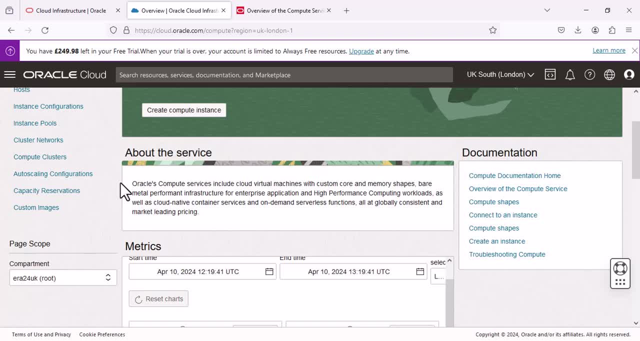 like 1 GB of OCPU and 1 GB of RAM, so don't go more than 1 GB or one CPU. so i see i have covered everything and now i have all these things. thanks for watching and stay with me on good health. have a nice day and good night, ilce, and hope that you have enjoyed this course. so se. all my aspects are clear. now say hello to everyone. thanks for watching till the end. you don't forget to likecomment and share it, and share it with your friends and help me with the future videos. so see you in next videoلك. So now i have all the homeland efficiencies in MyC mailек oneMs living room. up and find everything. 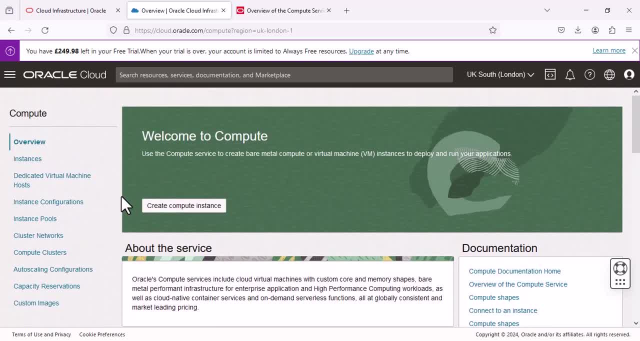 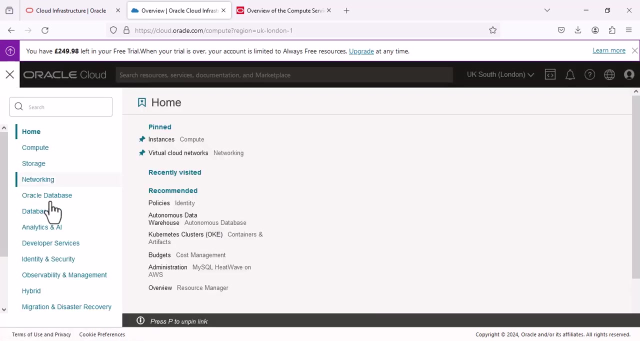 now i am leaving. now i am leaving them because it's hard for me to work like this way. i wasted my whole month checked everything, the databases i checked and, yeah, the all kind of information. but when the server is not installed, server is not ready, i cannot use the resources. whatever they are offering is useless. um budget cost. 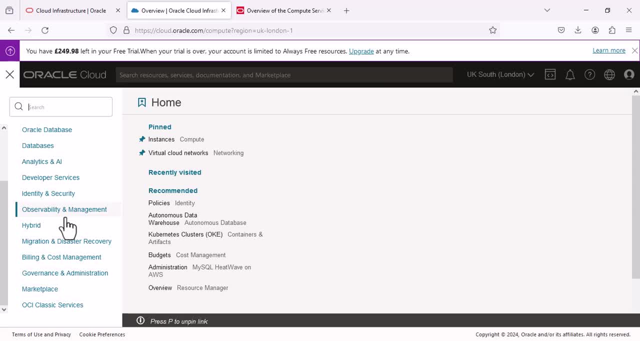 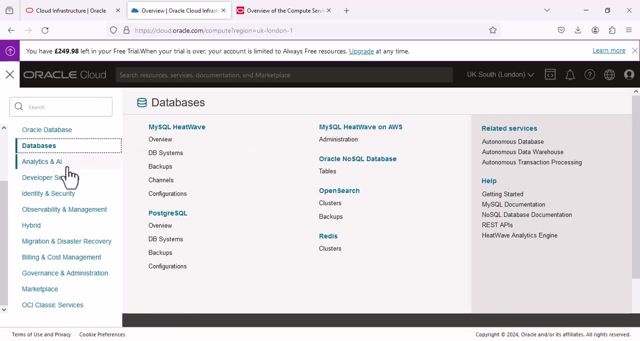 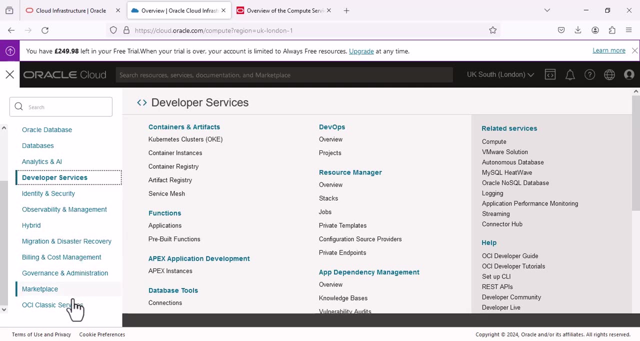 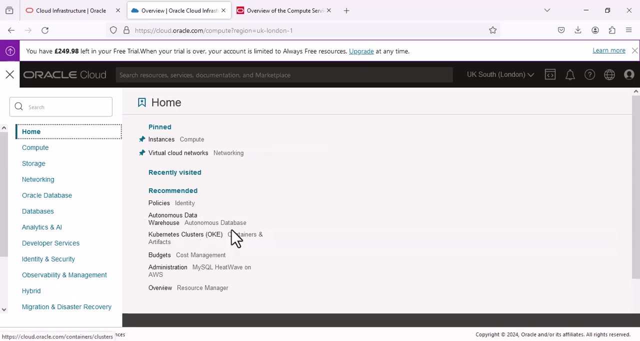 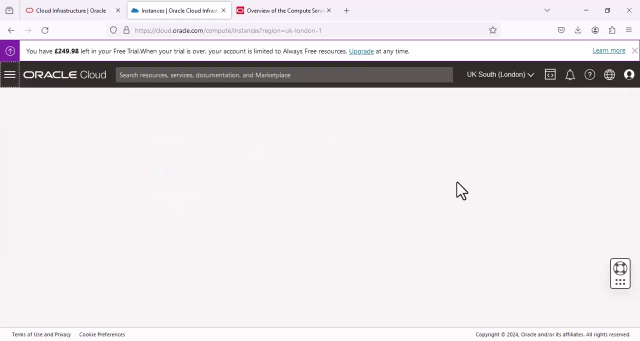 management. first thing. first, i need to have instance. instances are not available, so what i will be doing? um, i'll just have a look if i can cancel the tenancy, because uh, yeah, request tenancy deletion. yes, i think so, because so sorry, i'm not happy and it's useless for me, so request. 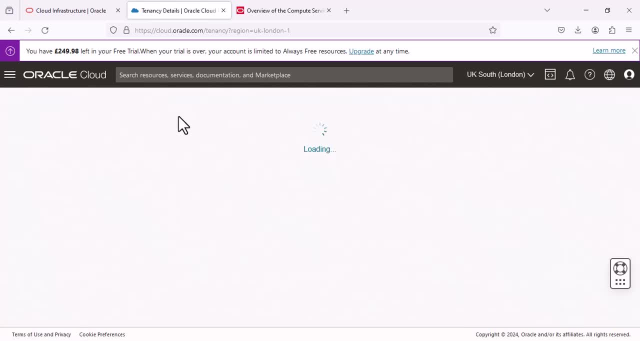 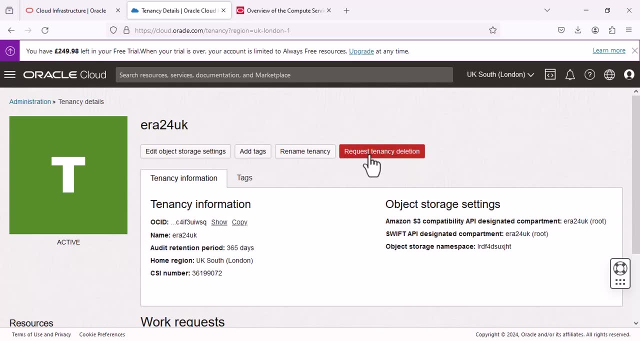 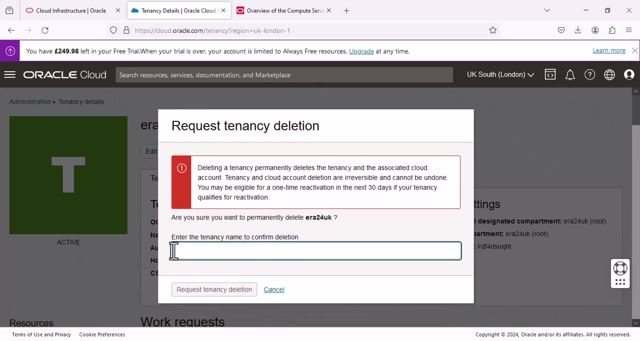 okay. deleting a tenancy permanently deletes the tenancy and the associate associated cloud account. tenancy and cloud accounts deletion are irresistible and cannot be undone. maybe um eligible for one time reactivation in the next 30 days. so if you want to reactivate your account, 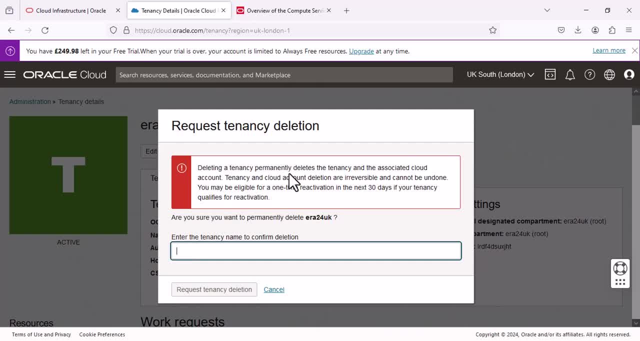 you will be able to reactivate in the next 30 days if your tenancy qualifies for reactivation. so i think we need to clean. i don't know why, but i think because i'm not going to practice on it and use as well, as they have no servers available. so i'm 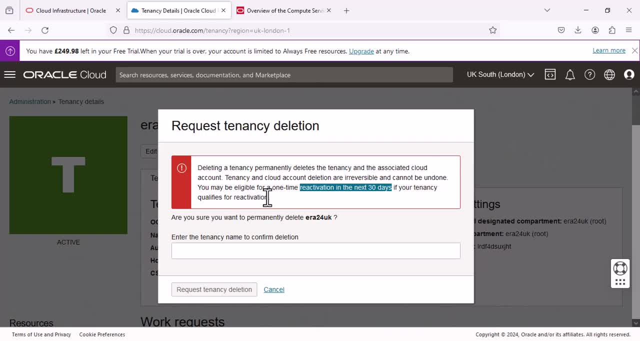 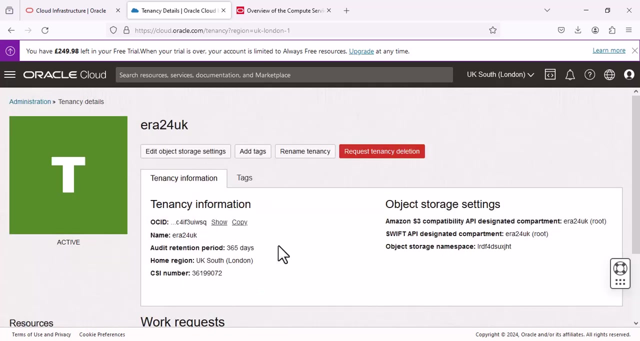 canceling now. oh, now you need to. you see another error. this error is saying the work request to delete your your tenancy could not be initiated. please try again and contact customer support. our order order request is being processed. I didn't put any order request. I don't know. that's full of error, full of errors and troubles. so, anyways, I hope.